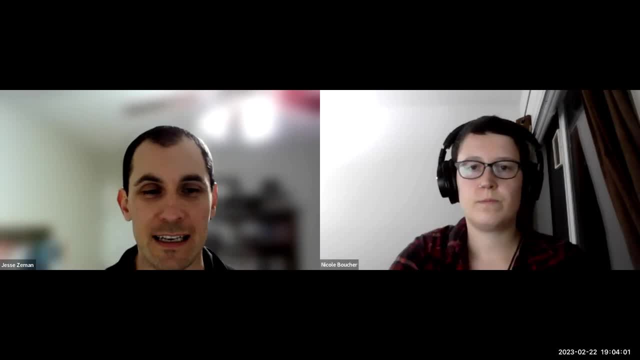 isotopes. After they completed their Master's in 2018, they started their PhD at the University of Victoria under Dr Jason Fisher and Dr Brian Strzomski. Their research focuses on how older moose calves are responding to landscape change from logging in the interior of BC with a 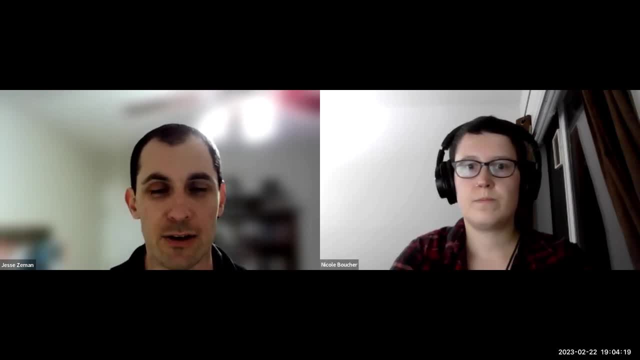 focus on the predation side of things. They currently live in Victoria, traveling to the interior to complete research around Prince George and Kamloops. So moose gets a lot of attention in the province. It's, you know, hits home for First Nations, for our members, resident hunters. 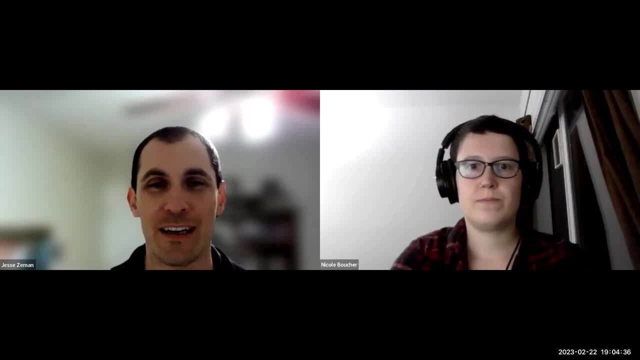 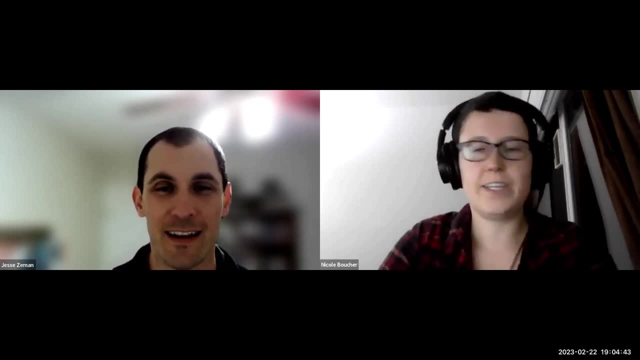 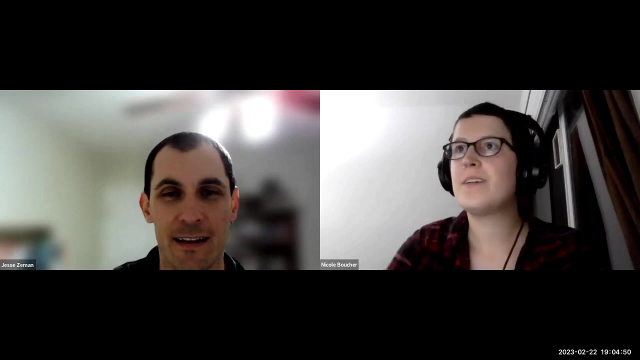 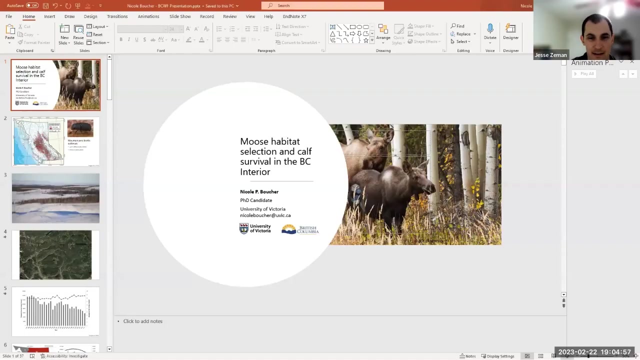 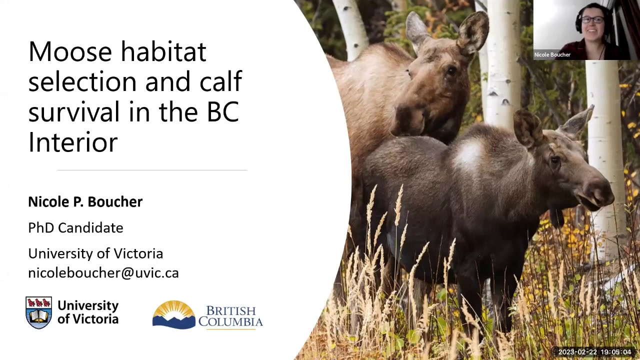 definitely a really important species. So, Nicole, we appreciate you taking the time to share what you're finding with us, and I'll turn it over to you now. Okay, thank you. Let's see if this works again, Okay, Or is that working? There you go, You're off to the races, Okay? So thank you for the introduction. 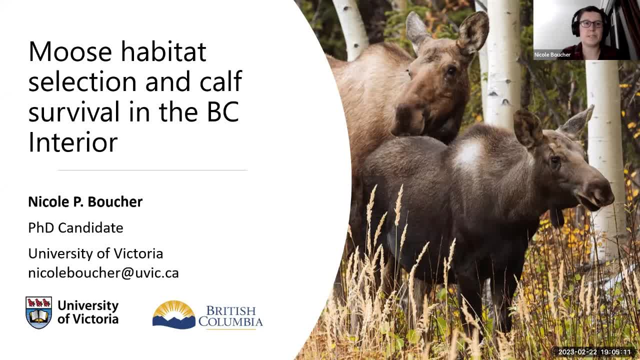 and, as you mentioned, I'm going to be talking about moose habitat selection, both from the mother's side of things, as well as the calf and how that relates to calf survival in the BC interior, particularly around Prince George and Kamloops. So first I'm just going to start off with a bit of a. 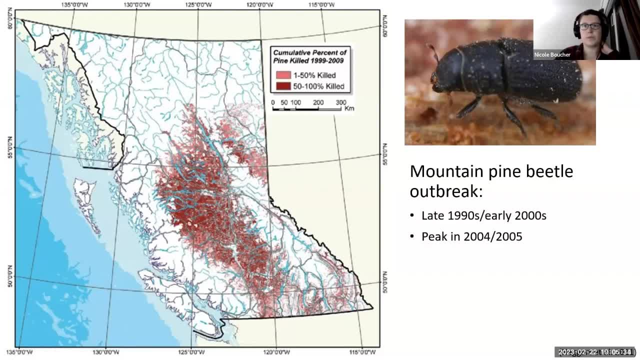 background about the landscape change and moose populations in British Columbia. So, starting in the late 1990s, interior British Columbia experienced the most severe and widespread outbreak of mountain pines in the United States. The moose population in British Columbia was a. 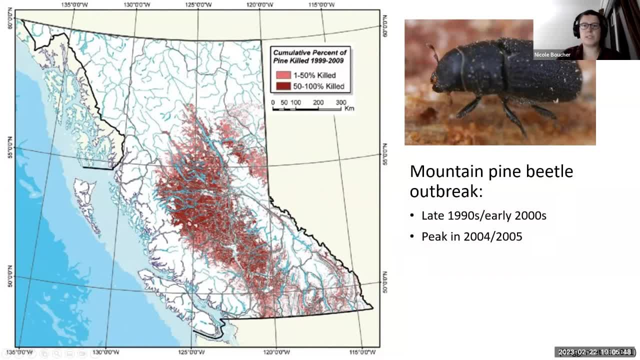 mountain pine beetle in its recorded history. So this massive outbreak followed several warmer winters which allowed more beetles to survive and led to larger mountain pine beetle populations which could overcome tree defenses, and so this led to a widespread outbreak where mountain pine beetles attacked around 50% of the total volume of commercial lodgepole pine in British Columbia. 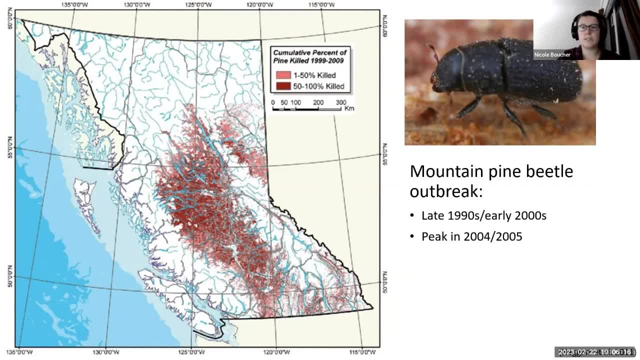 and the cumulative area of BCe-des-Hautaudes, the most active area of moose population on British Columbia of BC that was affected was estimated to be almost 20 million hectares, which to put into perspective, is about five times the size of Vancouver Island. So the most severe period of this outbreak was 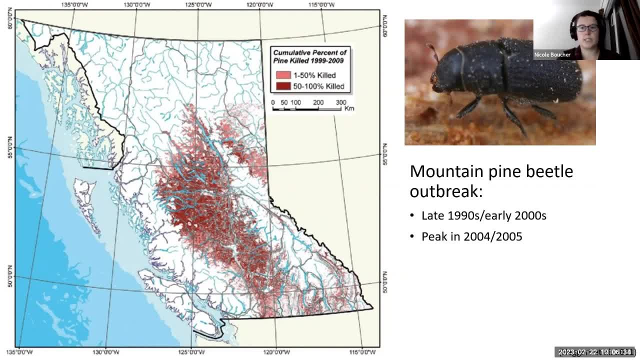 around 2004 to 2005,, with about 140 million cubic hectares killed that year alone, And while the amount of affected forest has declined since this, peak climate change is leading to Mountain Pine Beetle expanding northward. So currently a lot of our landscape change driven. 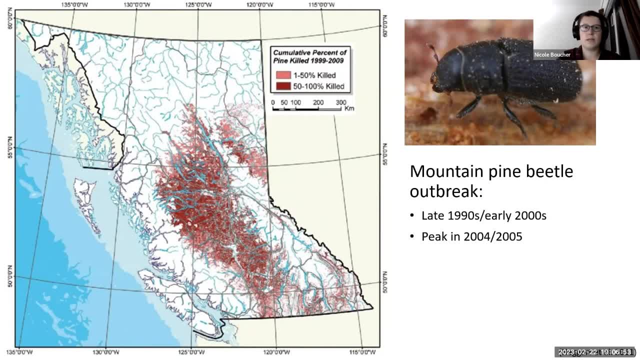 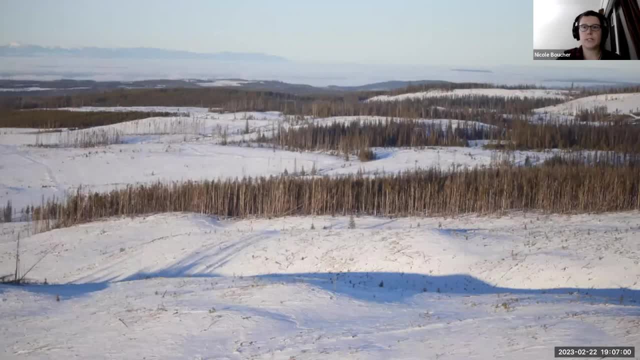 by this event is in the interior, but it will be pushing further north as winter is warm. So following the Mountain Pine Beetle outbreak, the BC government increased the annual allowable cut by 14.5 million cubic meters From the pre outbreak levels. so this was to capture as much economic value from the standing dead timber. 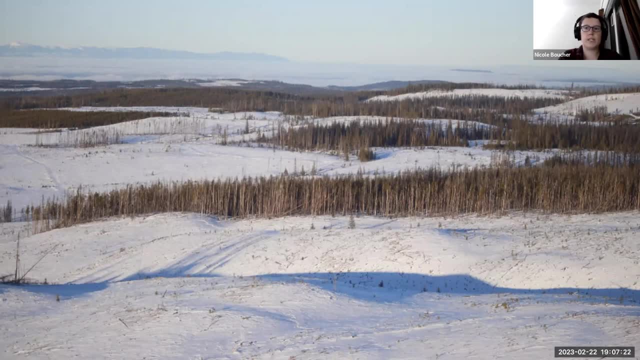 available as possible. So in many areas this more than doubled the annual allowable cut. This is in areas such as Vanderhoof or Connell, resulting in quite large cut block areas like the one shown in this photo. So this increase in timber harvest pressure has since resulted in patchworks of large cut blocks with tree 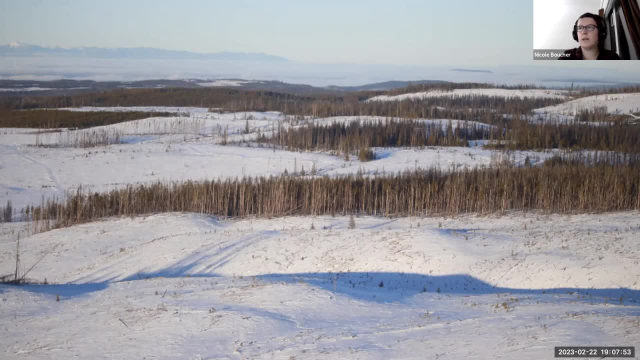 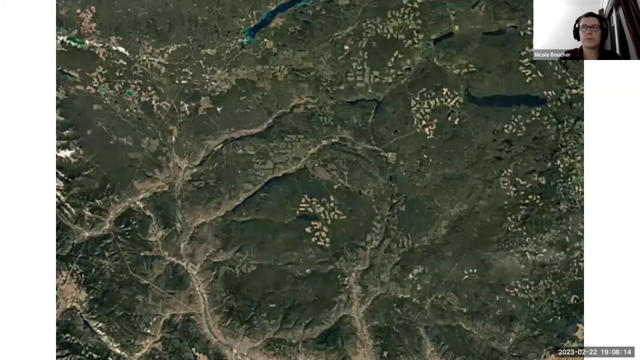 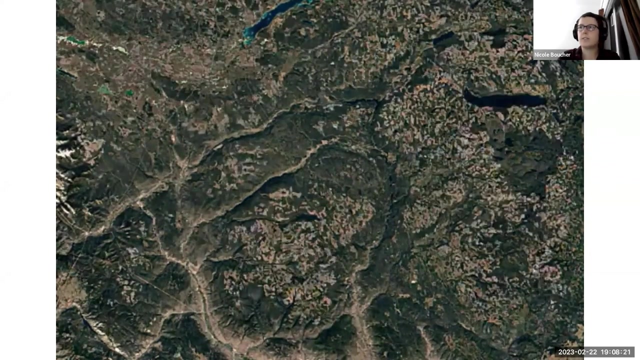 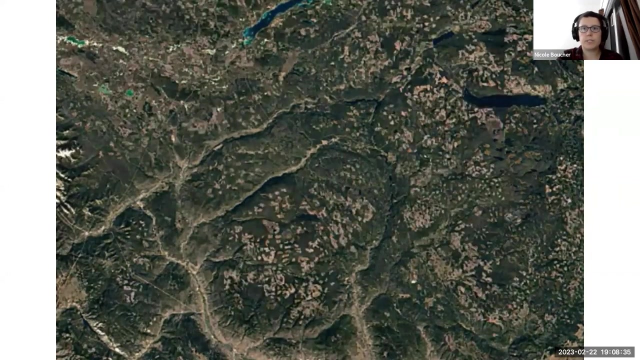 monocultures that are quite significantly managed And these are interlinked by an extensive network of linear features- just forestry roads- creating quite disturbed landscapes that are expected to have significant impacts on wildlife populations, Edmund. So this is just showing how severe these landscape changes being. 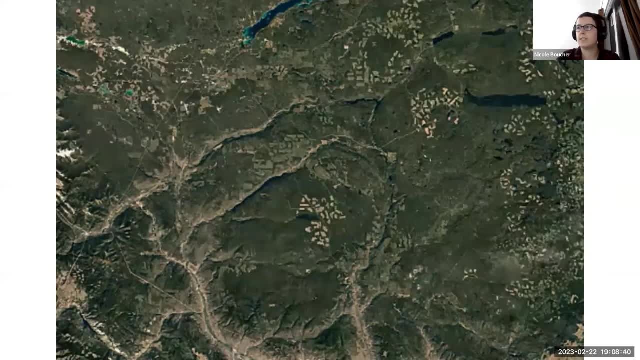 So, basically, this change happened from 1986 to 2016.. You can see that quite a bit of the plateau has shrunk and it is far more severe than it was in 2018.. Edmund, However, the main spchange hereو- 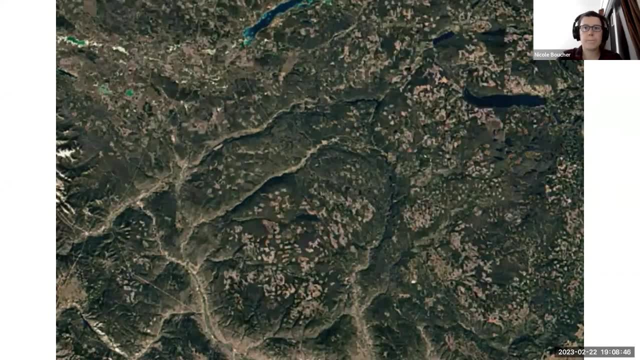 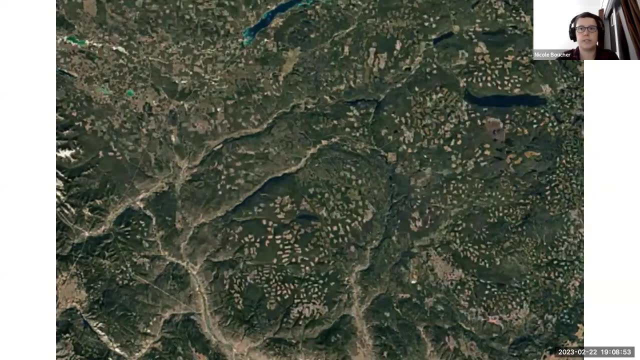 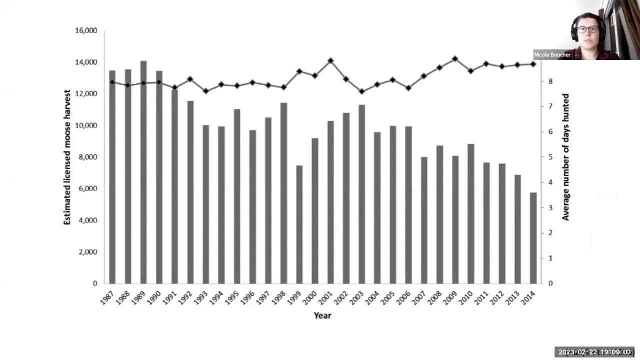 has been affected by cut blocks, and so the increases in annual allowable cut meant that timber previously allotted for logging in the coming decades has been harvested over just a few years instead. so this is a pretty drastic and rapid landscape change. So this coincided with increased timber harvest pressures across the BC interior, coinciding 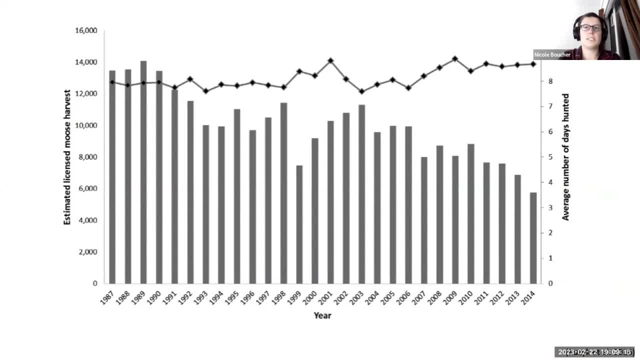 with the increased timber harvest pressures across the BC, interior Licensed hunter harvest most declined gradually by about half despite consistent hunter effort across the years. so you can see in this figure the bars are showing how the estimated most harvest, which is declining from 1987 to 2014, whereas the average number of days that hunters 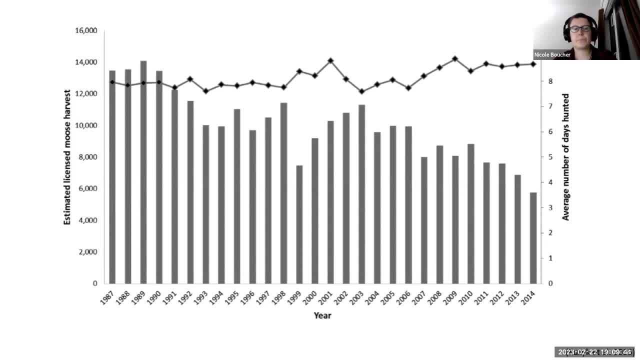 have gone out has stayed about the same. so the provincial moose numbers and harvests are pretty correlated. so this is suggesting that the declining harvest was a reaction to declining population trends and not changes in other factors like a hunter effort. so moose surveys conducted by regional 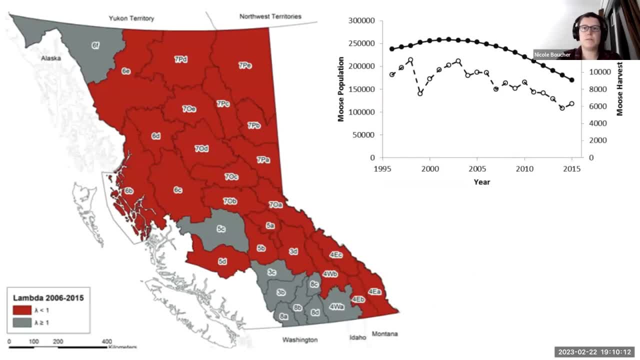 wildlife biologists during the winter of 2011.. So these are some of the changes that we've seen. So this is suggesting that the decline in population trends since the beginning of 2012 and through to 2013- 2014- suggested that population declines of 50 to 70% of moose had. 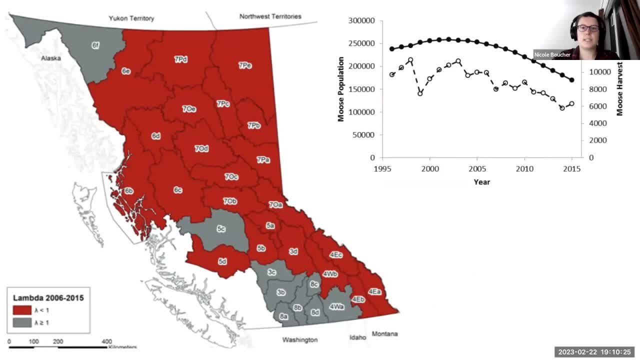 occurred in some areas of interior BC within the last decade. So from 1996 to 2005, most populations only declined in seven game management zones, so it's about 23% of the of the province, However, from 2007. 2000.. 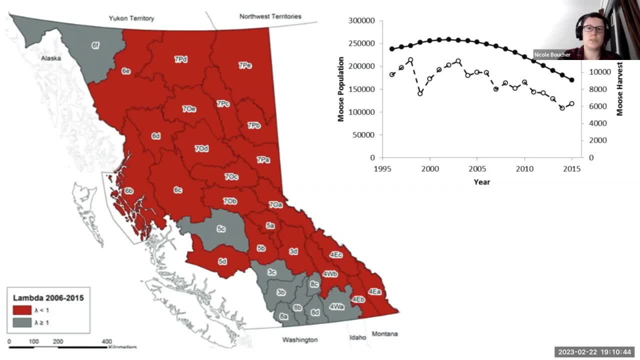 2006 to 2015, declines were found in 22 game management zones, so across 71 percent of the province. the model, the best models, including declining calf cow ratios, declining juvenile survival and declining cow survival. so overall, within this population study, the provincial moose population declined by 29 percent from 1996 to 2015, which is pretty drastic and, as you can see, 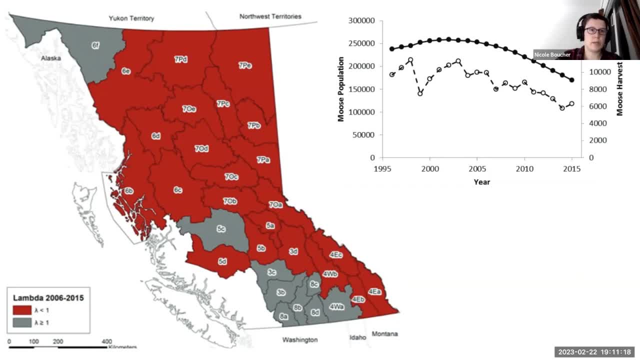 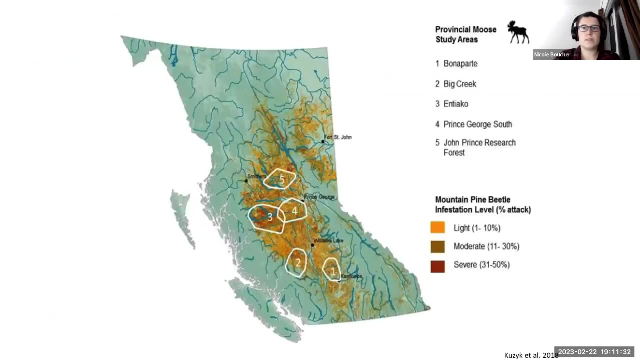 in this map, all of the red game management zones have a declining population during this time period, whereas the gray ones don't. they're either stable or increasing. they're gray. so the concurrent declines of moose with increased timber harvest indicate that a landscape change was likely a factor in moose population changes. 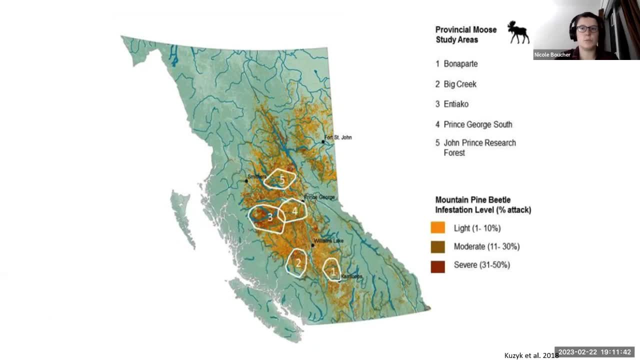 so, in response to moose population declines, the provincial moose monitoring project was initiated in december 2013. so the project monitored moose across five study areas and regions impacted by a mountain pine beetle across the province. so you can see in this map the five. 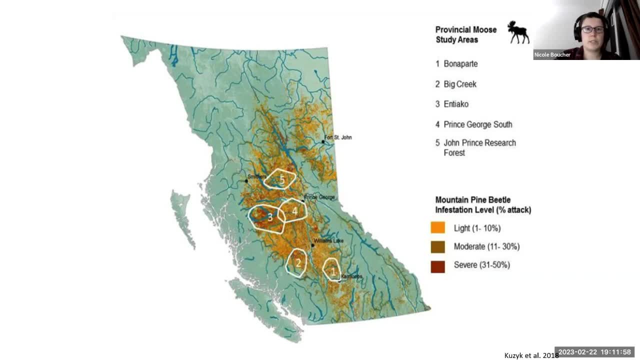 study areas are Bonaparte, Big Creek, Antiocho, Prince George South and John Prince Research Forest. they're spread across the province and the moose population declined by 29 percent of the total population from the maps of the 1850s to the mid-1950s. 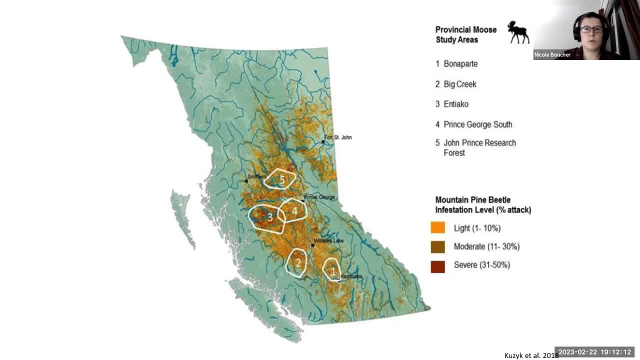 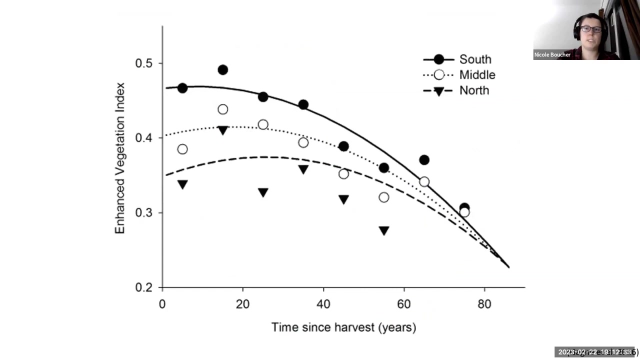 this is a different severity of mountain pine beetle infestation. so the orange to brown colors. so the provincial moose research project was hypothesizing that landscape change increased the vulnerability of most predators and hunters across the landscape. so following timber harvest, cut blocks, increase in vegetation, biomass increase in final crop growth and on average in most zoos we see more than丁ar's homines than in wild boar heaths and wild boars. 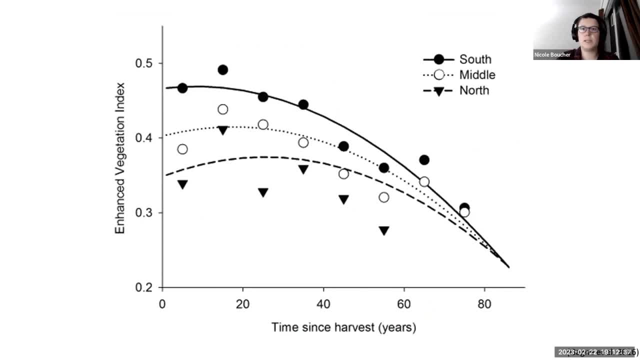 us quite rapidly peaking around a decade after logging, and this creates potential forage subsidies for moose, which can bolster their populations. similar to a wildfire, so the moose will tend to either increase in numbers after an event that creates more early cereal vegetation in the landscape, such as a fire or a cut block, either due to immigration or improved reproduction. 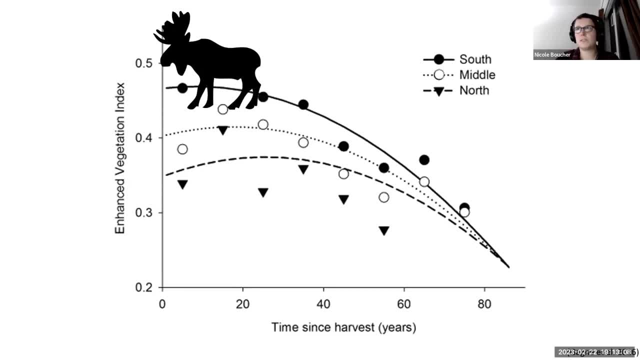 however, while cut blocks are often assumed to act similar to wildfire, there are some big differences that set them apart. so, for one, the forage and cut blocks may not be high enough quality or quantity due to sand tending practices that reduce forage, such as brushing or spraying herbicides, or 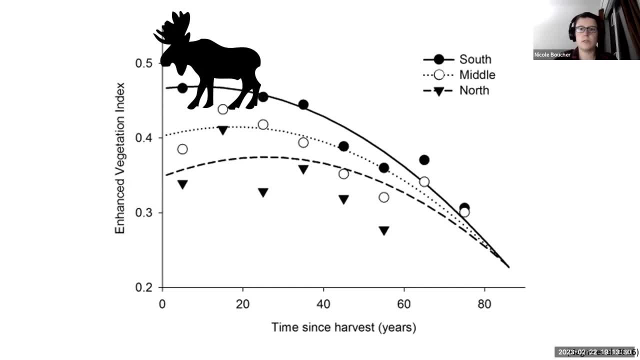 increased solar radiation. that increases secondary compounds. additionally, open habitats can increase stress of moose by reducing snow interception, which makes it harder for moose to move through their environments, and the open habitats also decrease thermal cover, which moose need to protect themselves from heat stress which they can get in both winter and summer. 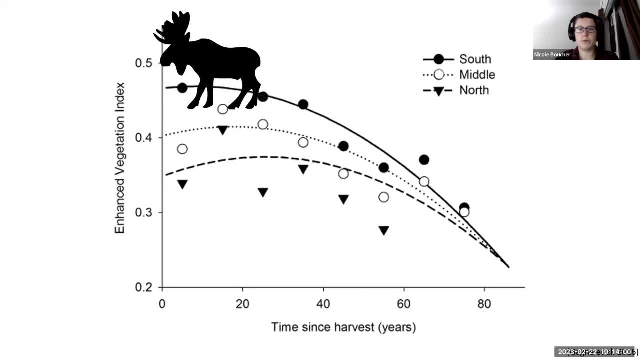 further. the logging can also create landscapes that improve predator and hunter search efficiency. results in landscapes that are much riskier for moose, either both directly through predation or perceived risk, which can lead to anti-predator responses that also decrease their, which also cause energetic stress. 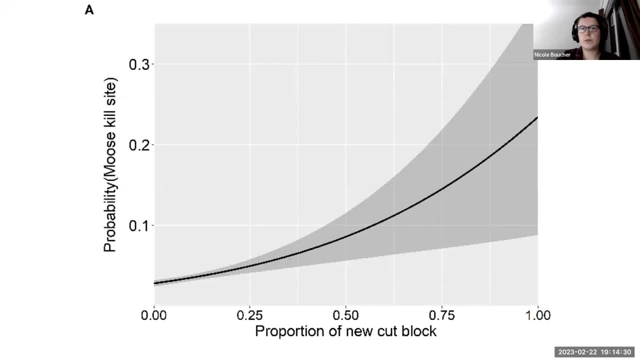 um. so there's growing evidence that anthropogenic modifications the landscape influences searchers' efficiency of predators and thus predation encounter rate, often by facilitate facilitating predator movement or increasing prey visibility. and this can be a problem, especially in the case for large-scale resource extraction, such as logging with large cut blocks that are linked. by linear features such as forestry roads. so cut blocks reduce hiding cover for moose, which can lead them to be more easily spotted by hunters and predators, and so, based off of some work that we did previously with colored wolves around Prince George, the wolf kill sites of moose are. 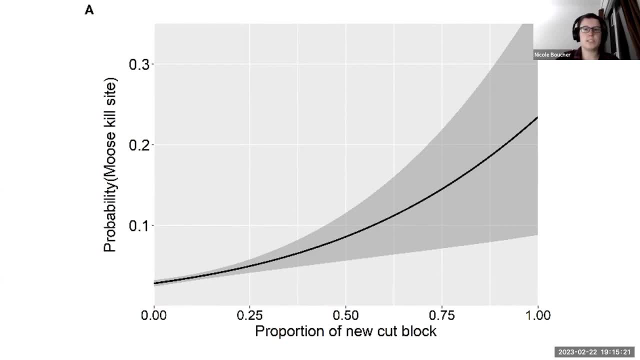 more likely to be found in new and regenerating cut blocks, suggesting that these are riskier habitat for moose. so, as you can see, as the proportion of new cut block and the landscape increases, there's a higher chance that you'll come across a moose kill site and while the 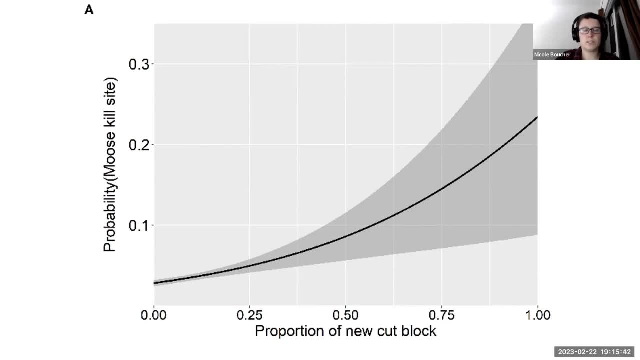 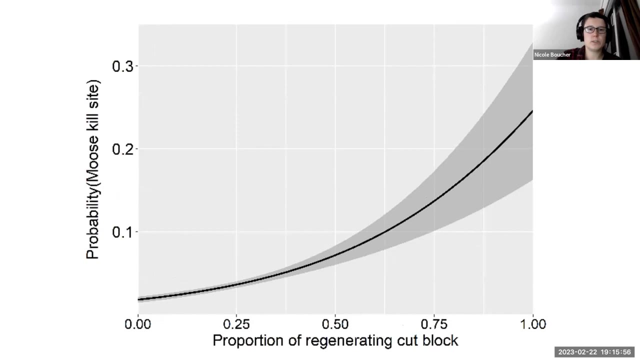 mortality site isn't necessarily linked to where the encounter of the prey would be, it does indicate that, potentially, these habitats are more risky and so, as you can see, the same pattern occurs for regenerating cut blocks having an increased chance of having a moose kill site. 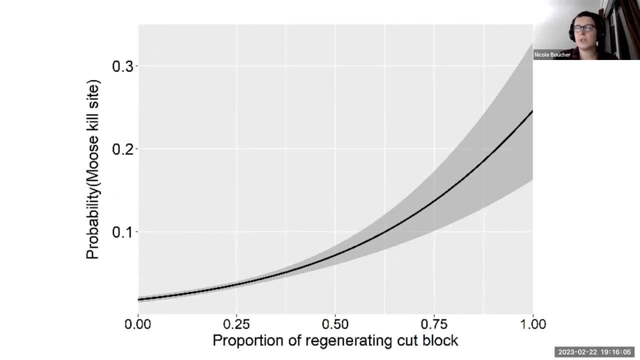 as well. data from the colored wolves suggested that wolves were selecting for younger cut blocks, which is possibly due to improved hunting efficiency, and they also moved faster in the younger cut blocks and selected for habitat that was closer to linear features. so this is consistent with previous research on wolf habitat selection. however, we also did find: 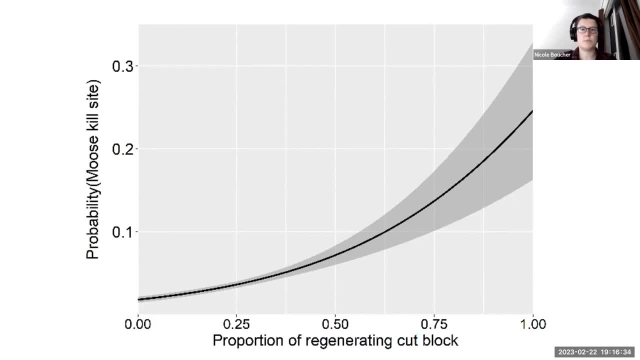 that linear features weren't an important predictor of moose kill sites, which indicates that linear features are mostly used as a travel corridor. so the combination of these two landscape features can mean that an area with both logging features connected by roads is pretty risky for moose. 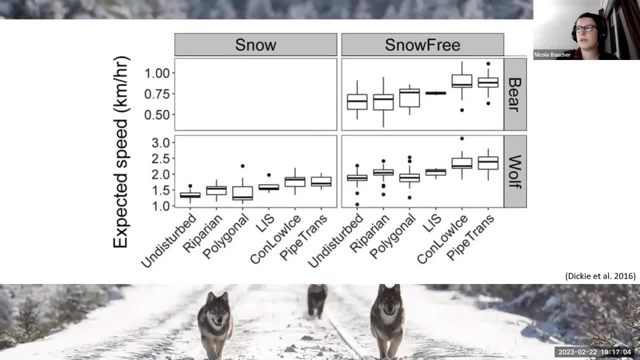 and this is supported by lots of other work on wolves, such as some work by melanie dickey- and looking at how wolves and bears move through their landscape, and their work found that the rate of movement for predators did increase quite a bit on linear features as compared to undisturbed habitat. 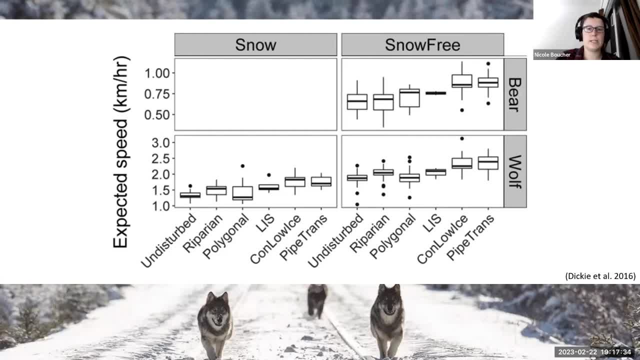 um. so this would um all adding up together, suggesting that the predators are using linear features to search moose habitat patches much quicker and further than in undisturbed landscapes as well. predators do often select for linear features, whereas prey avoid them, indicating that predators use them for moving, movement and hunting, whereas prey find them riskier, and this 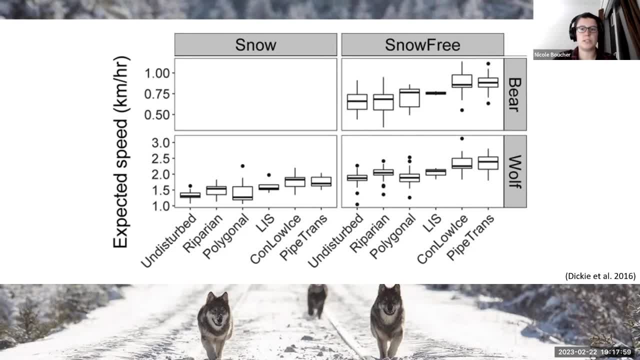 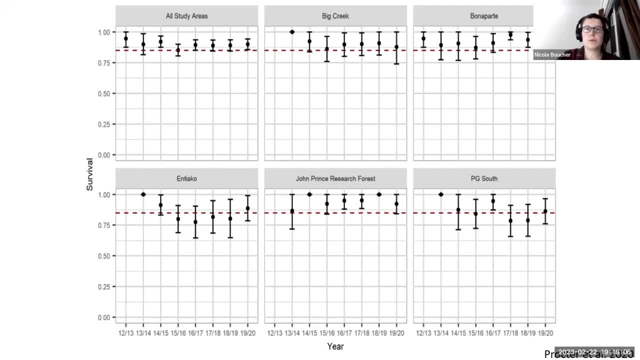 can contribute to declines in prey populations, where linear features are making prey more vulnerable to predation. um so the provincial moose research project expected that landscape change was increasing the vulnerability of moose by improving hunter and predator search efficiency, by decreasing hiding cover for moose and concentrating them in remaining patches. 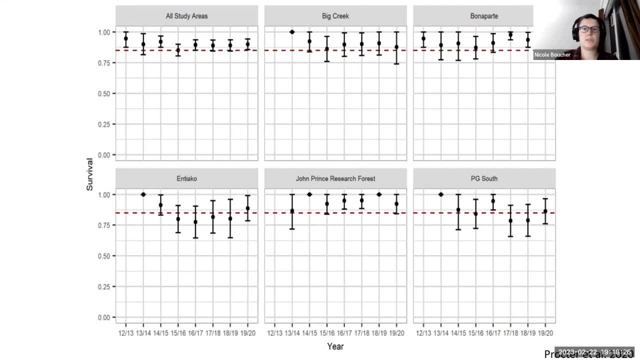 by also increasing uh energetic requirements due to reducing the vulnerability of moose, by increasing hunter and predator search efficiency, by decreasing snow interception by trees and reducing thermal cover, which would reduce body condition of recentering winter. and they expected that if their landscape change hypothesis was correct. 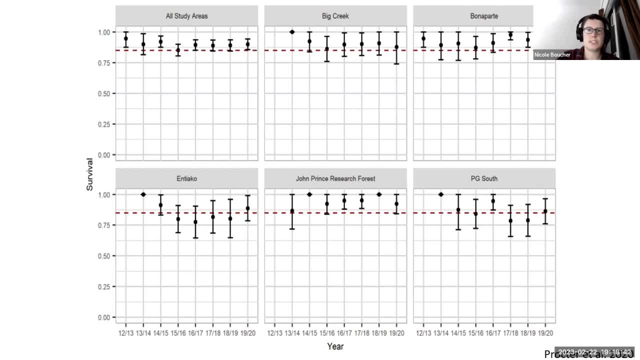 that moose population growth rates would be predicted to increase as cup blocks regenerated and roads were rendered impassable and moose were more evenly dispersed throughout the environment instead of being clustered in remaining patches. um as well, the um provincial moose research project expected that cow moose survival would have a greater 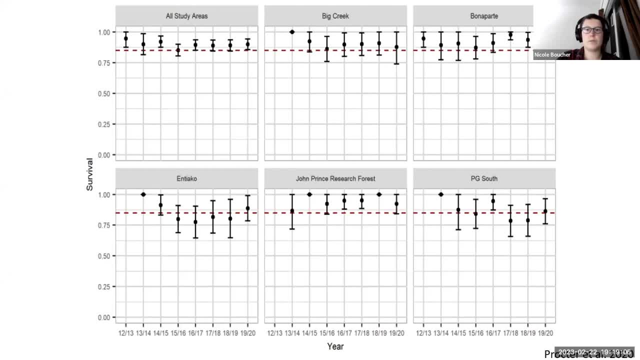 effect on population growth rates than calf survival did, because the declines occurred over such a short time period. however, when they did look at cow survival, the rates indicated about stable uh, the the survival rates were pretty stable and high um, which indicated that maybe calves were influencing population changes uh, more so than the cows um. so you can see in this figure um for 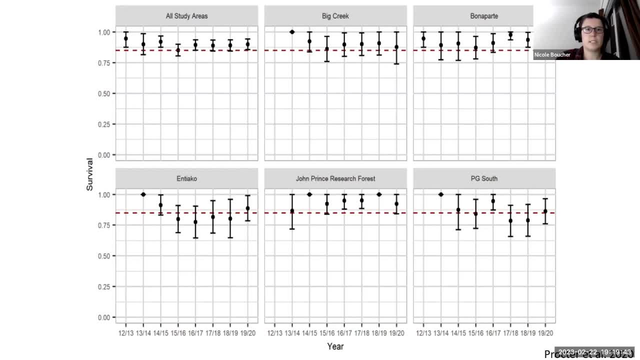 each of the study areas- big creek, bonaparte, antioch, oh john's prince research forest and prince church south um that generally cow survival across the years stays around um or above 85, which is required for a stable population, and while there are some years that 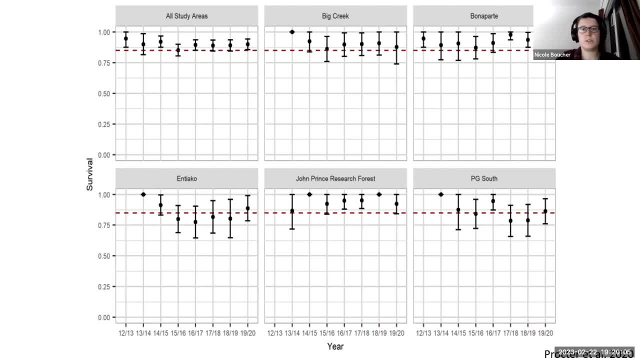 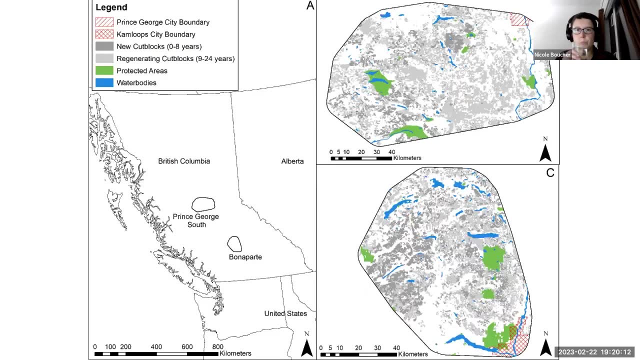 do dip below this kind of 85 threshold. generally they're above or their bars overlap um. so based on these results, the research project began coloring calves in two study areas, so in prince george south, which is south of couloir, and south of았는데, west of couloir. 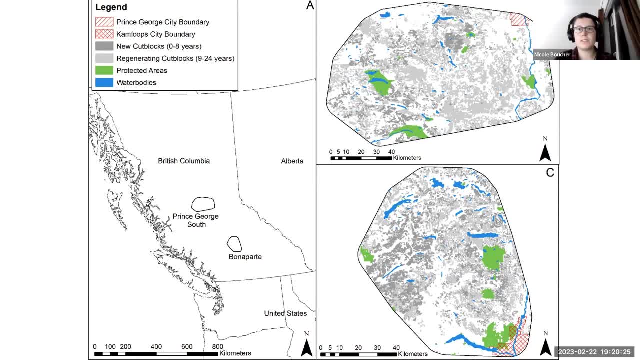 which is southwest of French George, as the the name kind of implies, and on the Bonaparte plateau, which is northwest of Kamloops. so in total, almost 200 calves were collared and monitored for body condition, habitat selection, movement and survival in both of these study areas. 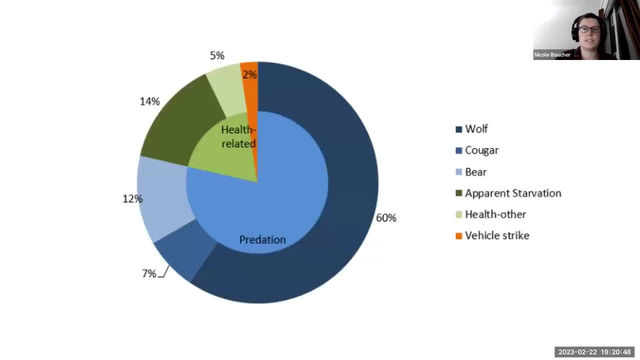 and, of these calves, most mortalities that occurred before one year of age were attributed to predation, whereas health related mortalities, which included apparent starvation, winter tick and other parasites or diseases, made up the other portion, because habitat selection impacts the exposure that an animal has to resources and risks. this led me to ask the question: how does mother and 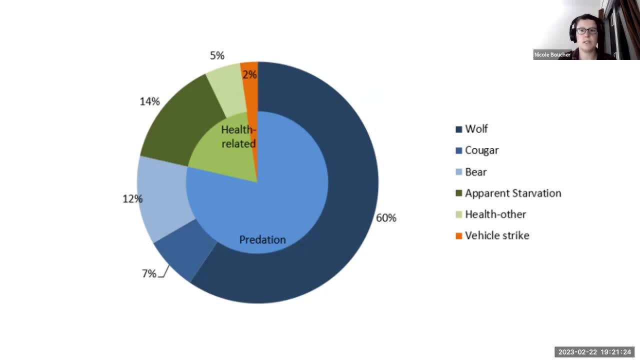 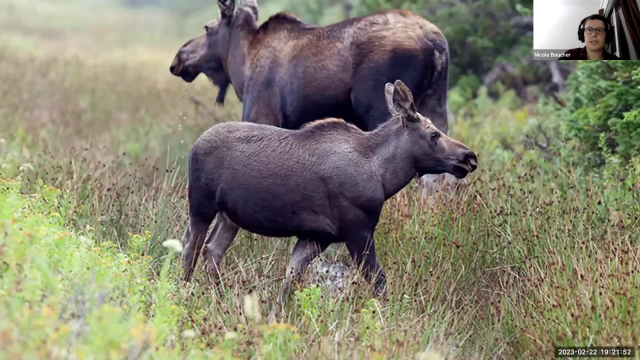 calf moose. habitat selection influence the survival of calves. because a large percent of the calves were dying from predation, i expected that either calves or their mothers were making poor choices. they exposed the calves to risky situations and led them to being predated on. because i was looking at older calves who are more independent, i decided to look at the habitat. 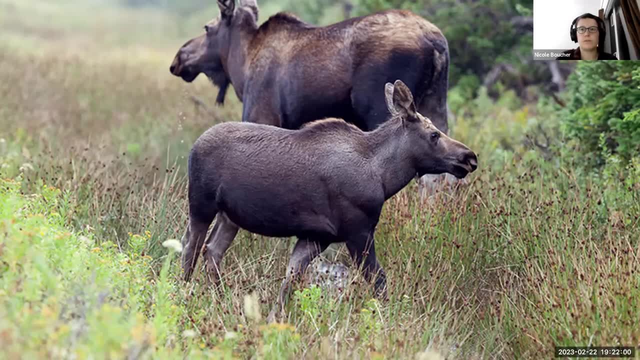 selection of both mothers and calves, so offspring survival is shaped by maternal habitat use at a young age, and when older um the calves own more habitat, selection choices play a more significant role. habitat selection impacts the resources and risks that animals experience, which consequently impacts the fitness of both. 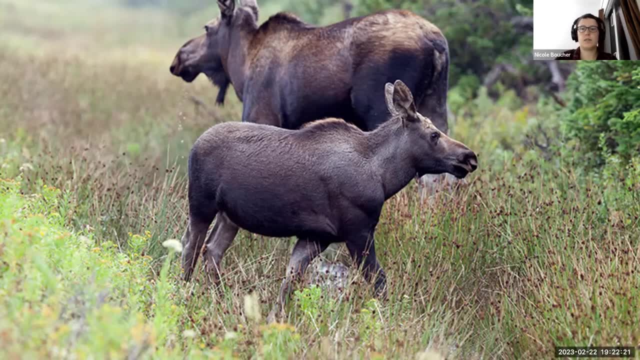 animals, and while females should select habitat that increases offspring fitness, these decisions can contradict what is best for the mother, and some others are expected to select for habitat that maximizes their net fitness, even if this comes at a cost to their offspring, and females must find the optimal maternal investment by balancing 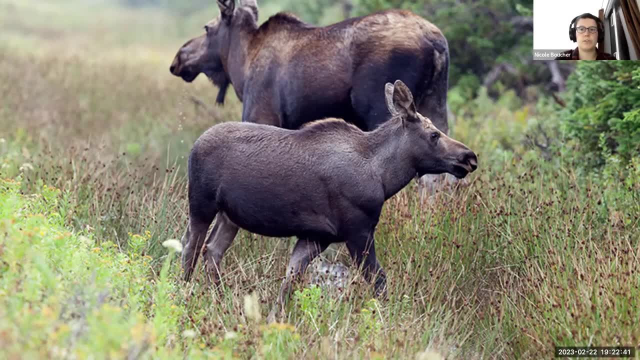 energy expenditure into current offspring with their own survival and future reproduction, and so when the calf is older and more independent, their calves habitat selection plays a more significant role in their own survival as well. so while calves are expected to make ideal habitat selection choices to improve their fitness, this isn't always the case. 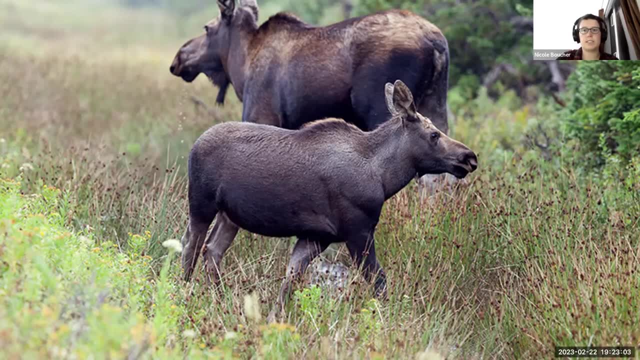 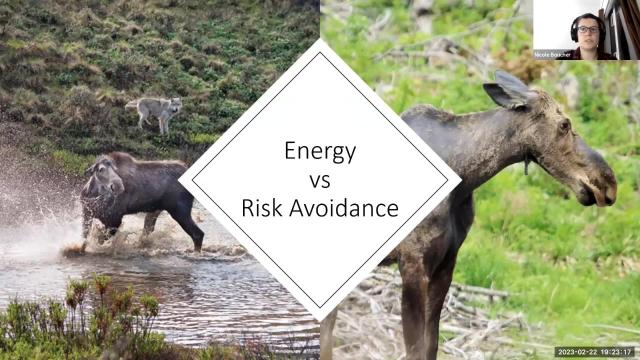 so calves are often inexperienced and they may make poor decisions that can lead to their own mortality. um and so. landscape change can make environmental cues more difficult for animals to interpret, leading to poor habitat selection decisions, and this can be more of a problem in inexperienced animals such as calves. and resource extraction alters the distribution of. 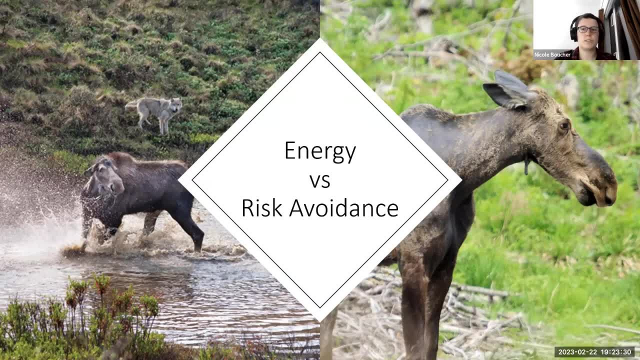 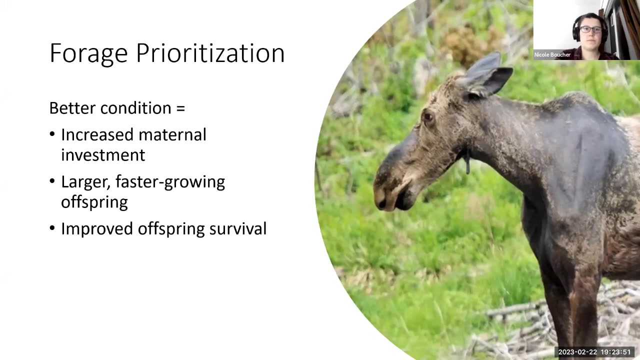 resources and risks to the landscape, which are both main drivers of habitat selection, and individuals make habitat selection decisions based on their own survival and risk angst against the environment. for example, animals are more likely to get in a bad habitat by age ten or more. that can, if a problem there is a problem with their survival. 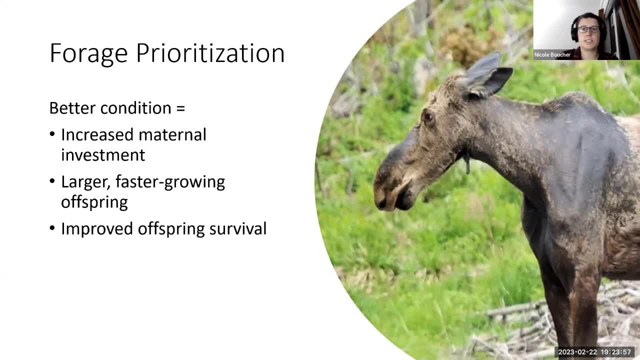 the residuals make habitat selection trade-offs between safety and resources based on their biological requirements, which impacts both reproductive investment into offspring by mothers, as well as both mother and offspring survival, or growing and healthier offspring with increased chances of survival for both the mother and offspring. and then the effects of malnutrition are both immediate and long lasting, such that 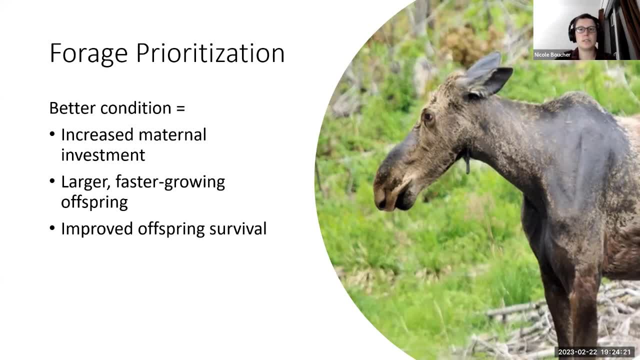 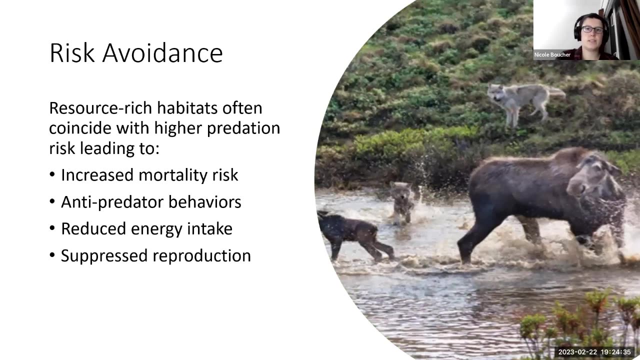 nutrition has lifelong impacts on the fitness of offspring, and this means that malnutrition, both prior to the calf being born and after parturition, can impact calf recruitment and, on the other hand, resource-rich habitat often co-occurs with elevated predation risk, so predators are expected to select for increased prey density, which should occur in higher quality. 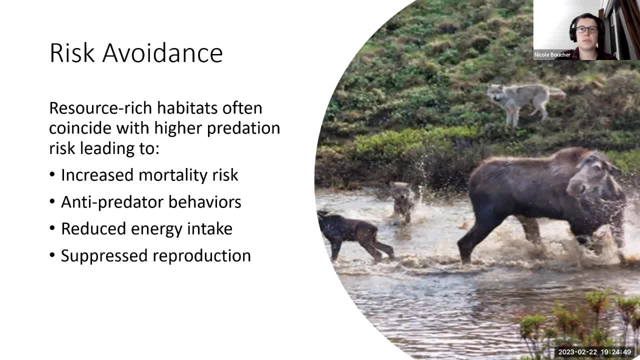 habitats and prey that select for these resource-rich but risky habitats have a higher probability of encounters with predators that could lead to mortality, especially for juveniles. additionally, increased predation risk may suppress prey reproduction due to anti-materials and anti-materials and so on. predator behaviors leading to poor quality offspring with smaller bodies, decreased body. 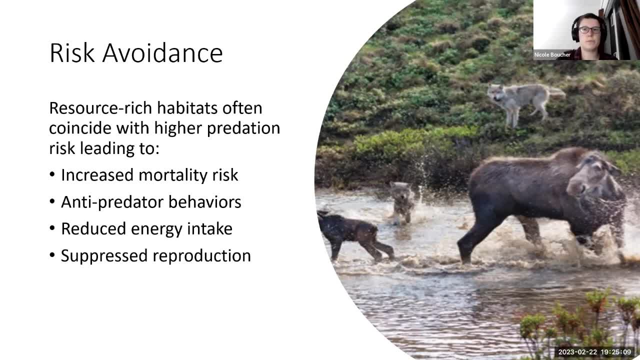 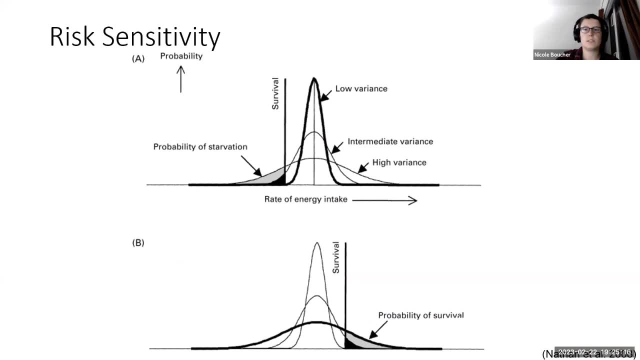 condition and increased probability of offspring mortality. so often, an animal's decision to avoid risk or prioritize forage depends on its internal state, so risk sensitive foraging theory predicts that animals with higher risk of starvation will take more risks, while animals in better condition will be more at risk adverse, and so this figure is showing how the rate of energy intake required 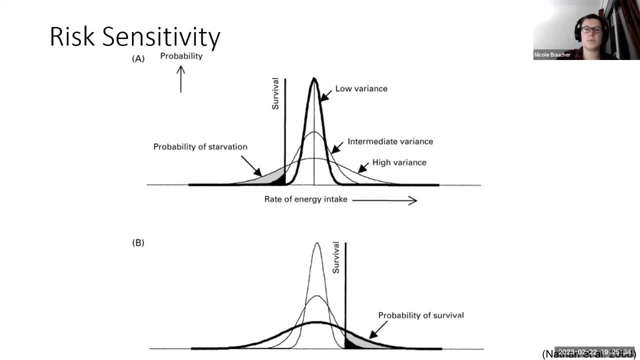 to avoid starvation changes depending on an animal's energy budget under varying food variances. so animals in good condition. so, for example, the top graph is showing an animal that's in good condition. they require a lower rate of energy intake to survive, whereas those in poor condition. 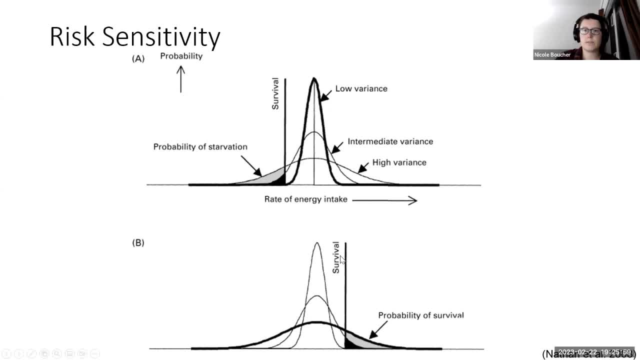 require a higher rate of energy intake to survive and have a higher chance of survival when they do take a riskier diet. so, basically, the habitat selection of animals in poor condition should reflect risk-prone behavior, whereas animals in good condition should avoid risk. those juveniles are highly vulnerable to limiting factors. these habitat selection 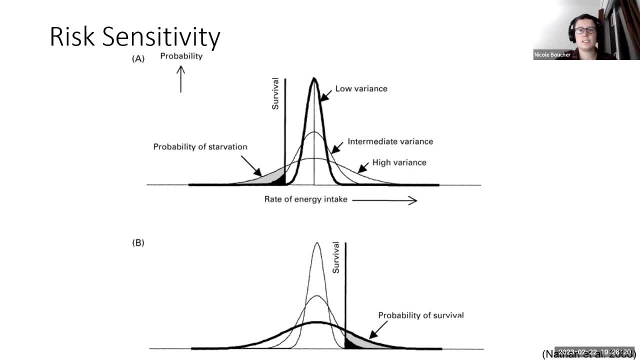 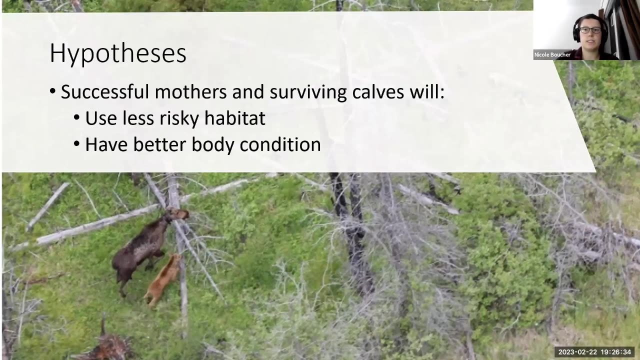 choices likely will impact survival significantly, and this is particularly pertinent in regions with drastic landscape change, such as interior british columbia. manager harim, my co-ousse Ved trying to find aren't you raft? and so we compared the habitat selection of successful and unsuccessful mothers and surviving. 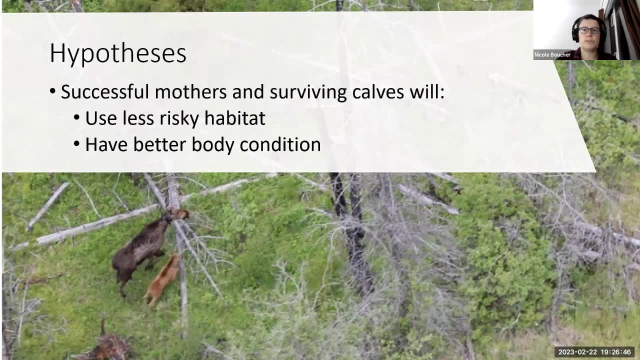 and non-surviving calves to determine how habitat selection in a disturbed landscape impacts calf survival. so we hypothesized that successful mothers and surviving calves would use less risky habitats. successful mothers and surviving calves would be in better condition and, as poor body condition does lead to animals making riskier decisions, which could lead to predation events of the calf. 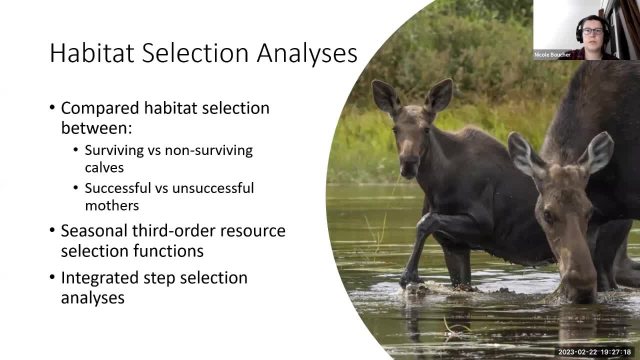 So to answer our questions on how habitat selection differed between surviving and non-surviving calves, as well as successful and unsuccessful mothers, we used two different types of habitat selection analyses, So I won't go too much into the details for these analyses, 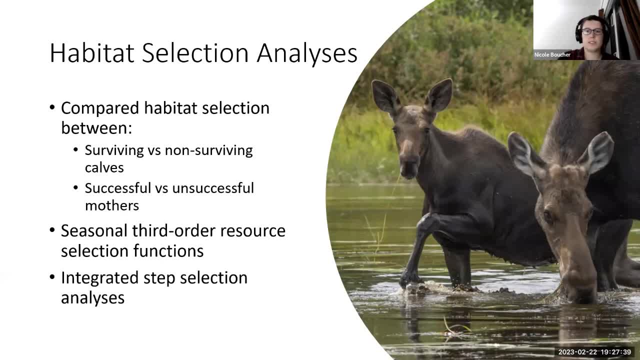 but for the mothers we used seasonal third-order resource selection functions which compared use to available locations within the animal's home range, and the mother's habitat selection was assessed for seasons both pre- and post-parturation, as maternal effects can be quite long-lived. And for calves we used integrated step selection analyses, which are: 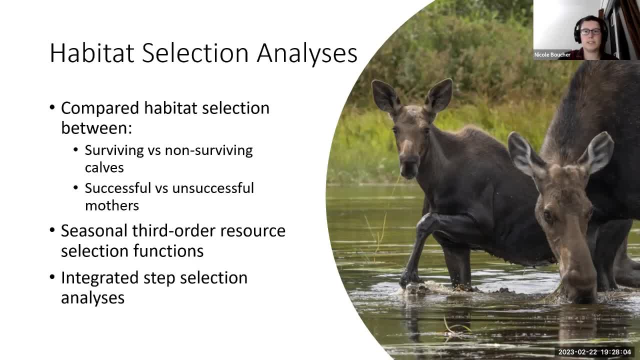 similar to resource selection functions, but integrate movement into the analysis, and these allow you to simultaneously examine both habitat selection and movement, while constraining your available steps to a more realistic sample of where the animal can actually move. And we were able to do this with the calf data because it had 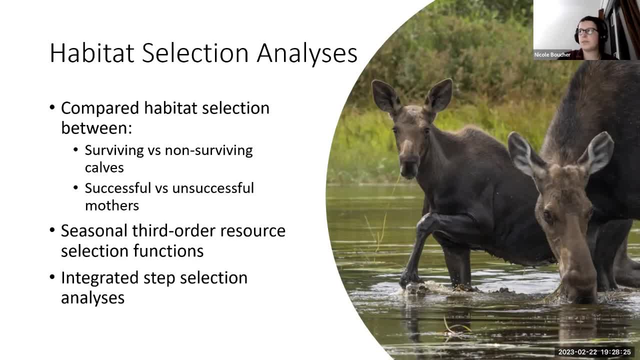 a finer, more accurate resolution than the adult female collar data. So for these analyses we defined surviving calves as living from capture to one year old and used the same designation for successful mothers, Whereas for non-surviving calves or unsuccessful mothers, the calf died between capture. 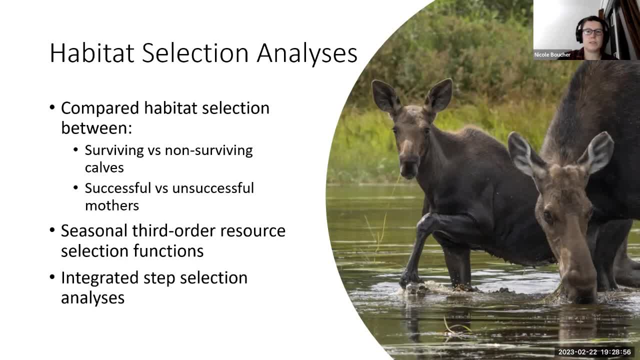 which was in January to March of the year, to one year old, which is around mid-May. So we looked at 187 calves for the calf analysis and 103 mother-calf pairs for the maternal resource selection. So we looked at 187 calves for the calf analysis and 103 mother-calf pairs for the maternal resource selection. 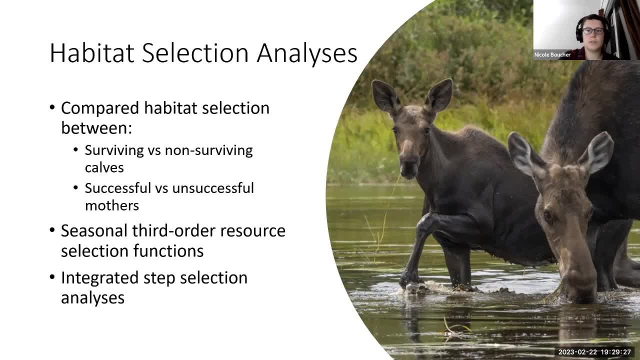 So we looked at 187 calves for the calf analysis and 104 mother-calf pairs for the maternal resource selection. And within the models for the habitat selection models we focused on And within the models for the habitat selection models, we focused on primarily disturbance features, including new and regenerating cut-blocks, linear features and Byrnes. 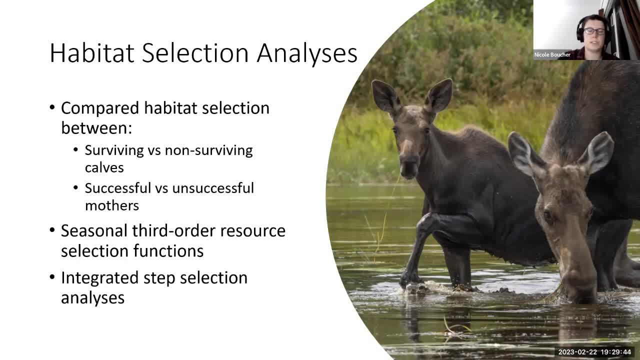 as well as other landscape features that may be important. forage or hiding cover, habitats such as forests and ponds am on tool which are supported. this tool is being Montgomery Park equivalent choir. these are other documentary INFORM. mare wollte phrases such as farm industry is still in the curriculum and still want to все. 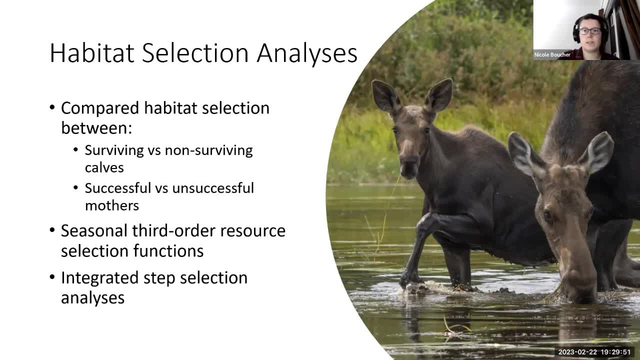 or quite close some not Avatar- science on sensors, technology, competence at short term, carbon detection and possibility of idols- omehoyeattformINGING also one of the top rotors. Vielleicht this is part of the research on largeATT. to do some real Richter isn't really for Georgia all right. 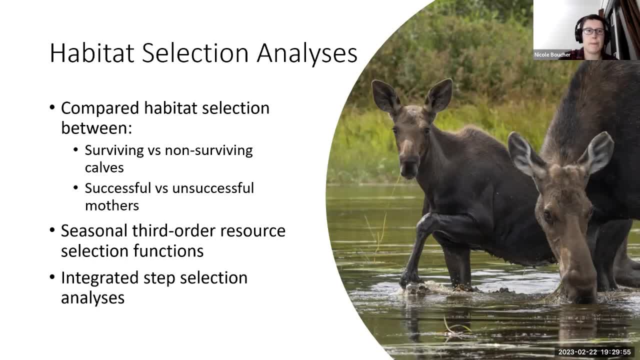 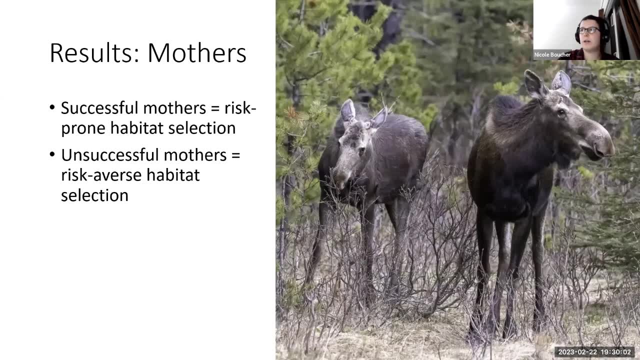 such as forests, water bodies and topography. So start off with the results from the maternal analysis. So, converse to our hypothesis, we found that successful mothers appeared to adopt a more risk prone habitat selection strategy, whereas unsuccessful mothers appeared more risk adverse. 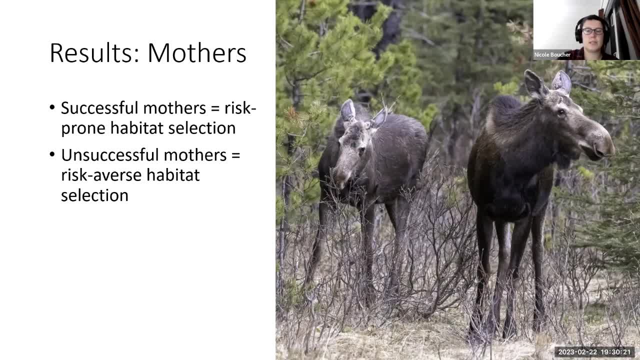 So successful mothers selected for early serial habitats such as young cup blocks and burns, which would provide more forage. They also exhibited reduced selection for forests, as offspring vulnerability decreased, And then unsuccessful mothers, on the other hand, selected for habitats with lower foraging potential. 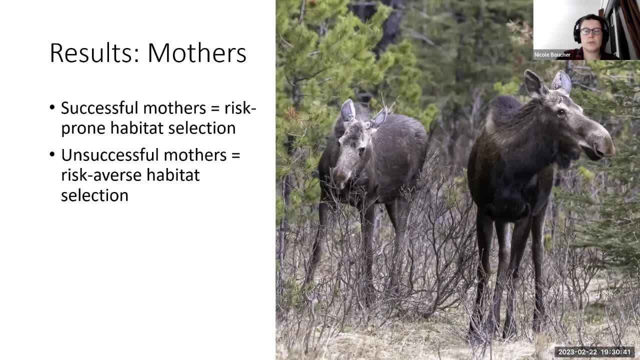 but more cover, such as forests, And we also observed consistent selection patterns for certain features within regions, indicating that all mothers did perceive certain spatial features as good or bad habitat. So, for example, both successful and unsuccessful mothers showed avoidance of habitat close to linear features. 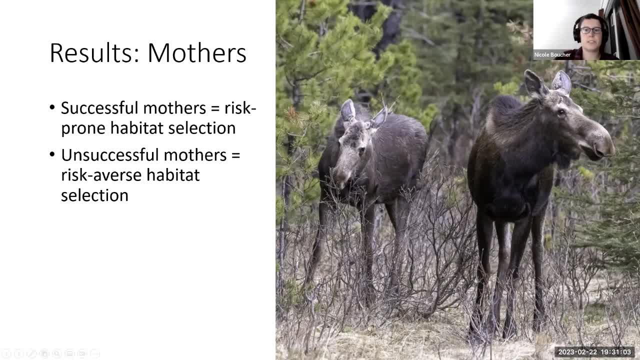 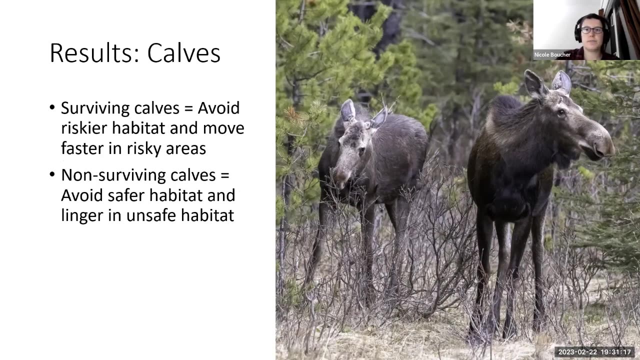 and with high linear feature densities, And they also all seemed to select for edge habitats which would provide hiding cover For the calf analysis. we found that the habitat selection and movement of calves in disturbed landscapes varies between regions that you look at, as well as recruitment statuses. 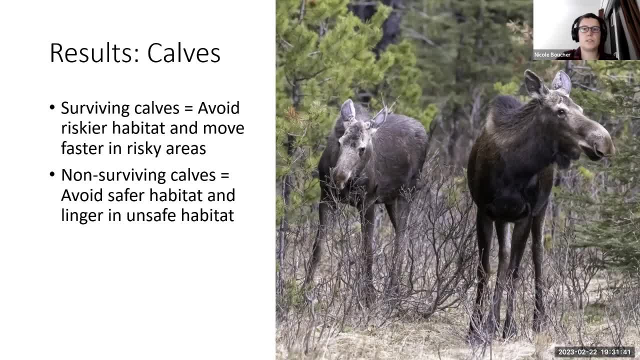 So the recruited calves did appear to avoid riskier habitat and move faster when they were in risky areas. So, for example, surviving calves selected for habitat with more hiding cover, such as regenerating cut blocks, water bodies and forest cover, And they also moved faster near linear features and open habitats. 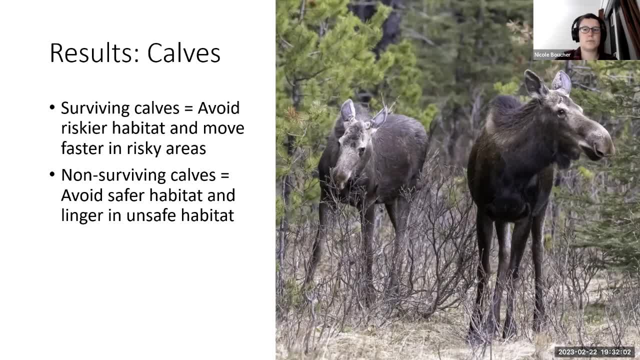 While non-recruited calves appeared to avoid some risky habitat, they also appeared to avoid safer habitat and linger in unsafe habitat, possibly due to foraging, which could have increased their predation risk. For example, they moved slower in new cut blocks. 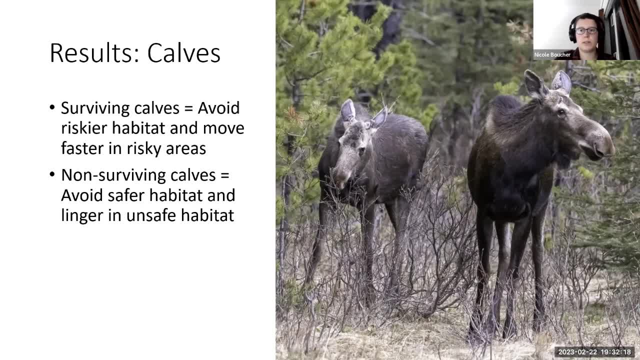 and avoided escape habitats like water bodies or high elevation habitats. So, for example, they moved slower in new cut blocks and avoided escape habitats like water bodies or high elevation habitats. So, for example, they moved slower in new cut blocks and avoided escape habitats like water bodies or high elevation habitats. 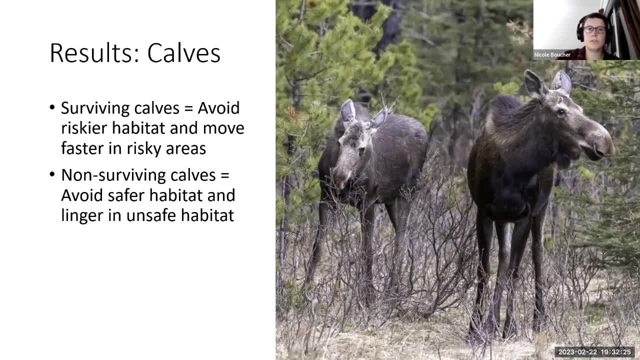 And some of the results found to be somewhat light. in kind of for these results, I've highly simplified them because the analyses were quite complex. So if anyone is interested in kind of a more detailed breakdown, feel free to email me. just my first and last name: evic dot co. 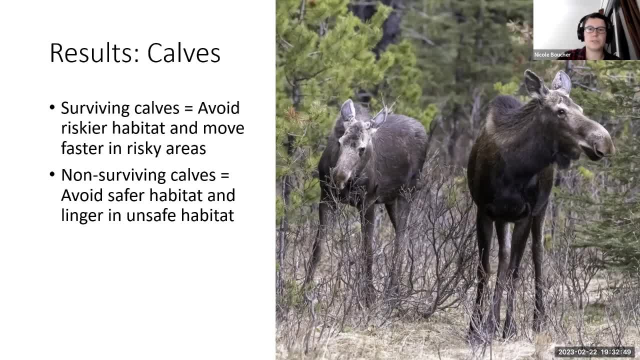 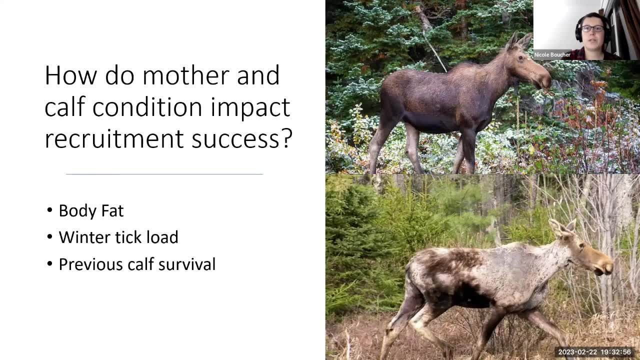 I'm happy to go into more detail. It would just be a little bit look too confusing for a presentation, um. but our next step, um was asking: how does mother and calf condition impact recruitment success? um. so we expected that variation in habitat selection between successful and unsuccessful females would reflect maternal quality, with unsuccessful females 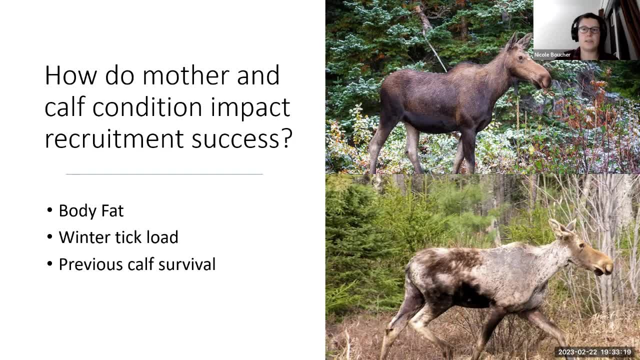 being in poor condition, with lower body fat and a higher tick load, and having lower success with their previous calf. and for the mothers, we looked at both current and legged measures for body fat and winter tick load, so we did limit the analyses with the mothers that had been captured twice in 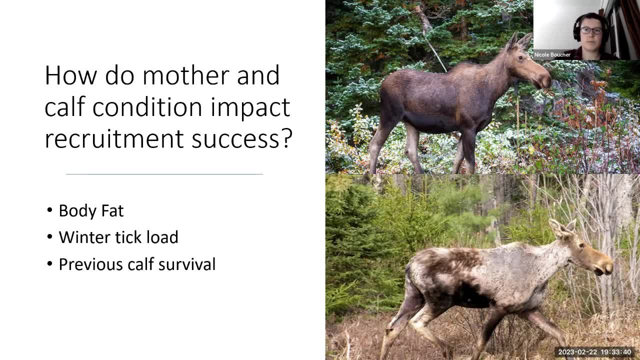 consecutive years to allow for the the legged measures. and then we also compared calf body weight and winter tick load. and then we also compared calf body weight and winter tick load between surviving and non-surviving calves. so we expected non-surviving calves would have a lower. 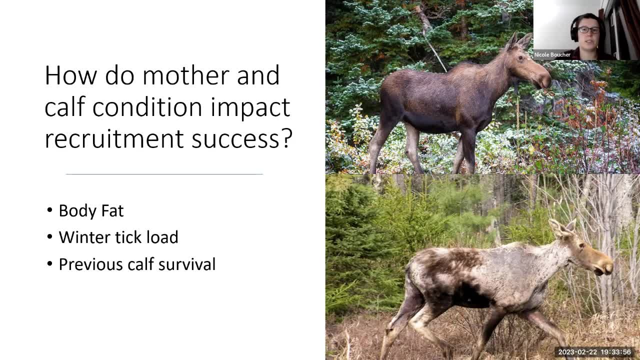 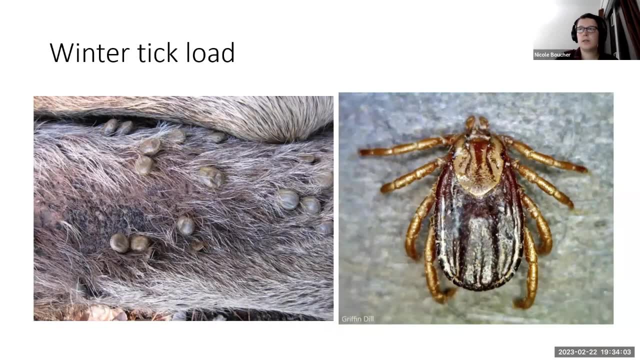 body weight and higher winter tick load, putting them in a worse condition and more vulnerable to limiting factors. um. so winter ticks um attach onto moose uh through the winter and they they quest in the fall and attach um stay attached through the winter before dropping off in the spring. um. and while attached uh winter ticks on heavily infested. 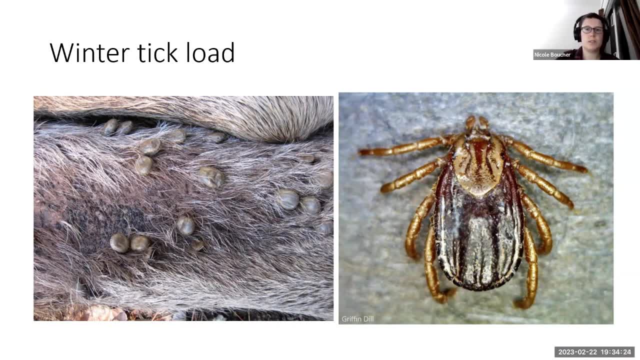 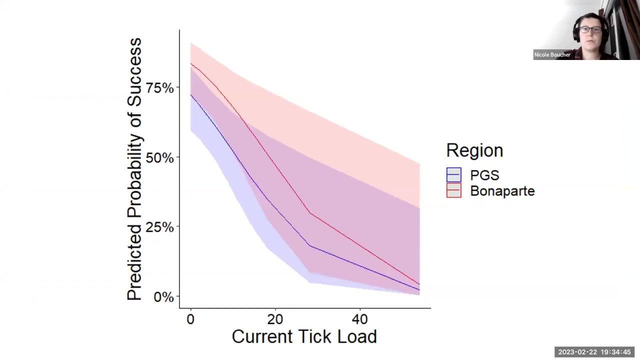 moose will take huge volumes of blood, and this blood loss requires significant energy to replace and can have quite a significant impact on moose health, leading to things like hair loss and even mortality due to the energetic stress induced by the infestation. so So, when looking at mother success, we found that female moose success did decrease as 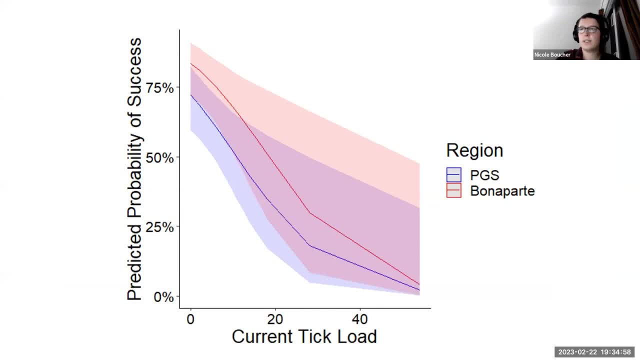 their tick load in the current year increased. So basically, the cows with higher infestation likely had less energy that they would be able to infest into their calf, leading to a higher chance of calf mortality. However, we found that the legged winter tick load, so the winter tick load in the year 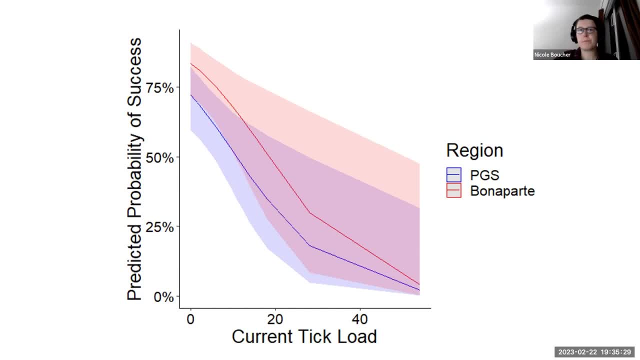 before the calf was captured was not significantly related to the mother's recruitment success. So these results show that female moose success decreased significantly as their tick load increased. The results made it surprising that unsuccessful moose were adopting a risk-adverse habitat selection strategy, which we would have expected, so this possibly contributed to reduced energy. 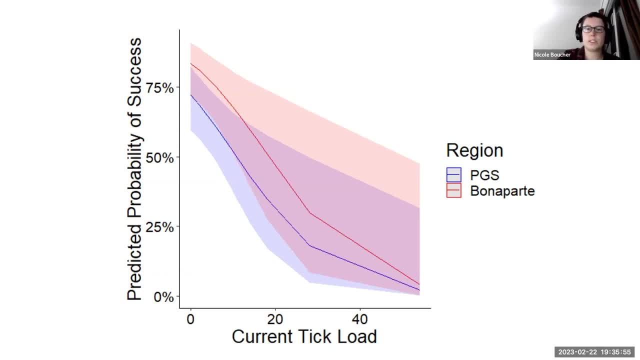 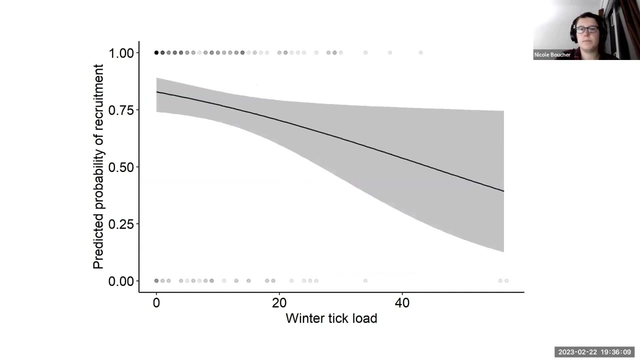 allocation to offspring. Additionally, offspring of unsuccessful females could be exposed to habitats with higher winter tick densities, leading to increased calf infestation. For calves, we found that As winter tick load increased as well the probability of recruitment decreased. So this matches the results from the maternal analysis, which found that unsuccessful females 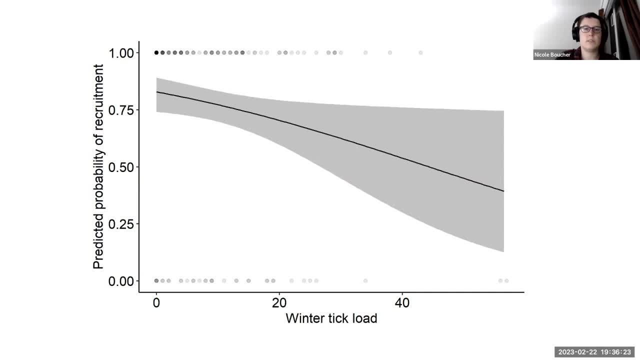 had higher winter tick loads, So likely the non-surviving calves get a double whammy of having higher winter tick loads that reduce their energy, potentially also having mothers that are contributing less energy allocating into their offspring, Leading to reduced calf survival. 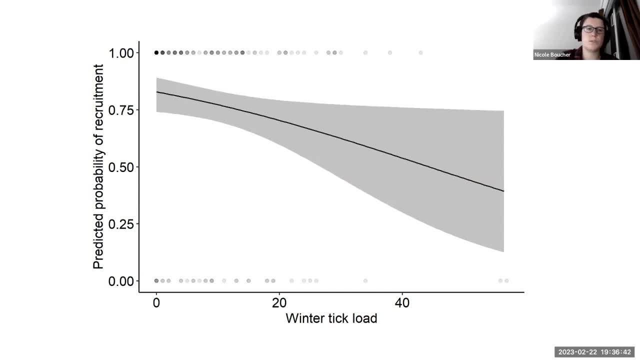 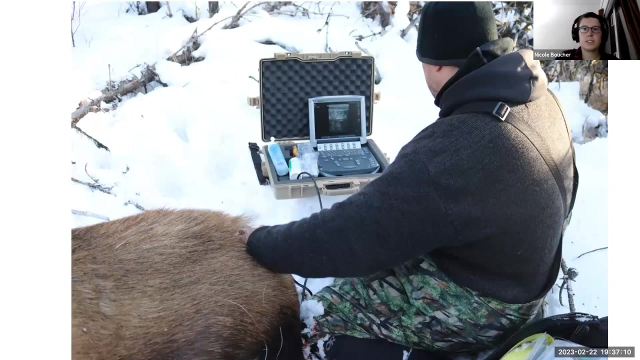 So these results were expected, because winter ticks do have a quite drastic impact upon moose calves, And some calves do have quite significant winter tick loads which would be expected to lead to their mortality. Next, we looked at the relationship between body fat and mother success. 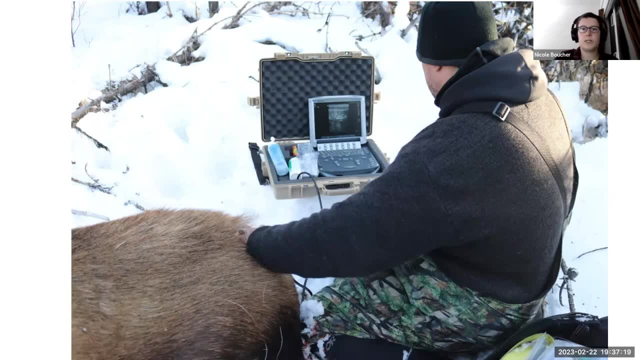 So we measured the maximum rent fat using portable ultrasounds as a measure of mother body condition. So this was done during the period that the mother was captured And we looked at both the current body condition as well as the previous year's body condition. 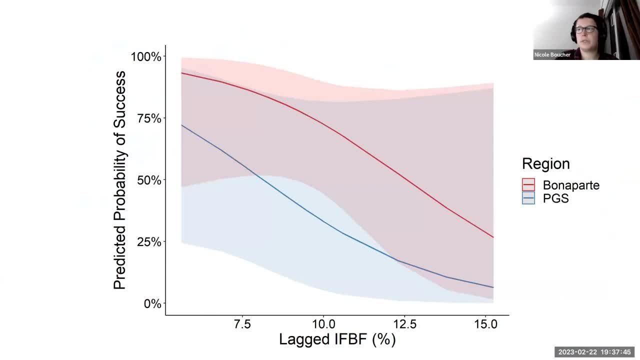 So, surprisingly, we found that the probability of mother success in recruiting a calf actually declined with increasing body fat in the previous year. However, the mother success was not significantly related to current body fat, So this is unexpected, Because we would assume that a mother that was in better condition or who had more body 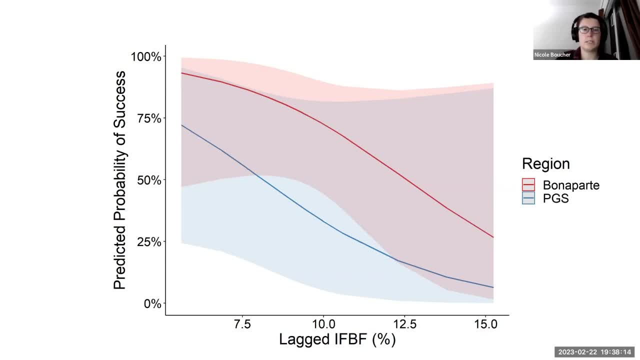 fat would be able to allocate more energy into her offspring as well as make less risky decisions. that would contribute to potentially higher recruitment success of the calf. So, while we expected the successful mothers would have a better body condition, there wasn't, And this doesn't appear to necessarily be the case. 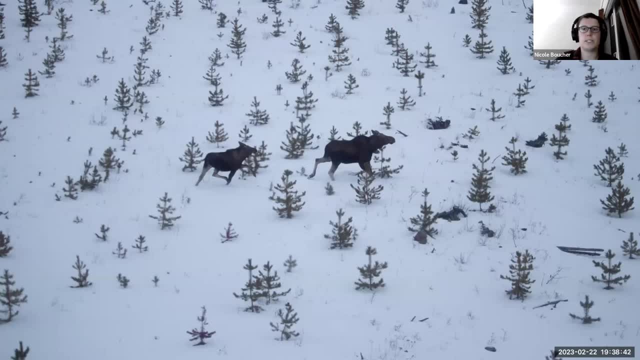 So our next step was comparing previous calf survival between successful and unsuccessful mothers. So this step was completed using data from midwinter aerial surveys, which we completed the year prior, as an estimate of whether females were accompanied by a previous calf in the year prior to calf capture. 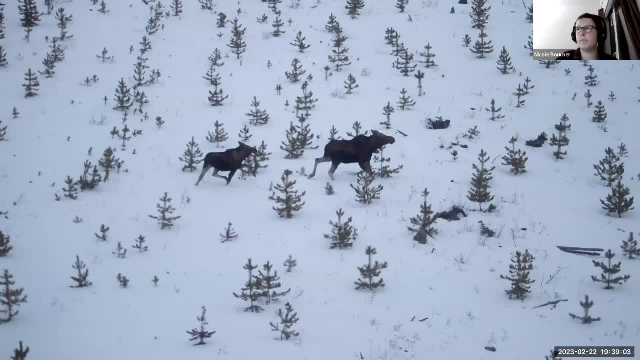 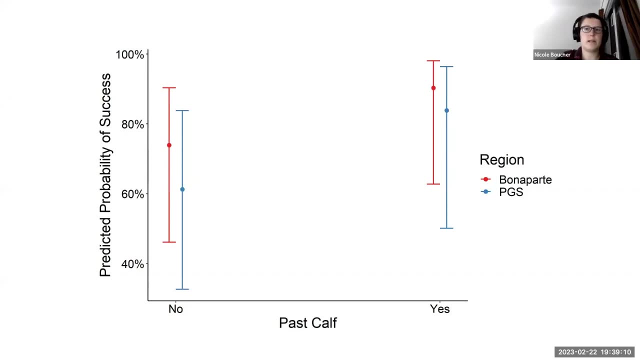 So this is looking at. Okay, So we found that mothers with a calf present midwinter had a higher probability of being successful the following year. So successful mothers may just be better at keeping their calves alive, And this may also explain the decrease in probability of success for mothers as their 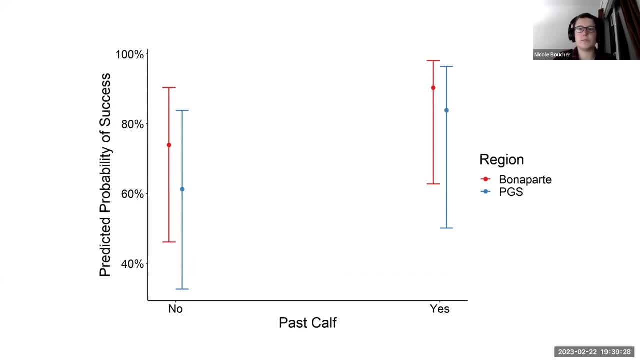 body fat in the previous year increased, So successful mothers would have been accompanied by a previous calf, Which would have led to reduced body condition due to diverted energy resources, whereas unsuccessful mothers were not burdened by a calf, So they would have been able to invest all that energy back into themselves, and which 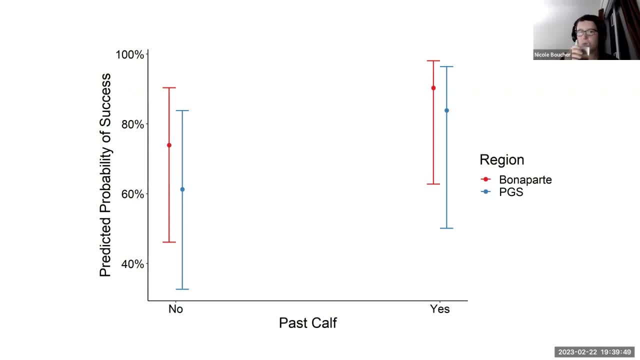 would have led to a better body condition. So this analysis also indicates that successful cows are potentially more consistent with their calves. So this analysis also indicates that successful cows are potentially more consistent with their calves. So this analysis also indicates that successful cows are probably more consistently successful. 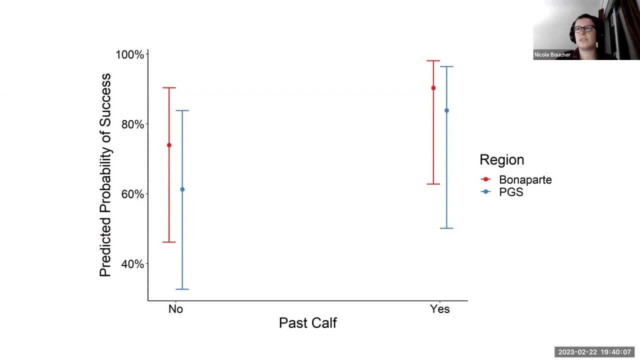 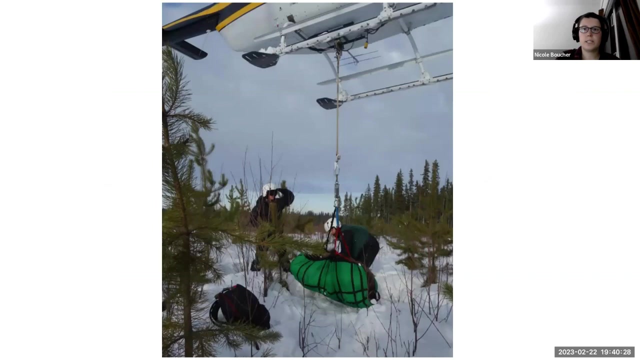 So something that they're doing, something that they're doing- is seeming to be working better, Although we do need to follow the emails for more than just two cows to get a better look at whether this is actually the case or not. So the last thing that we looked at was we compared. 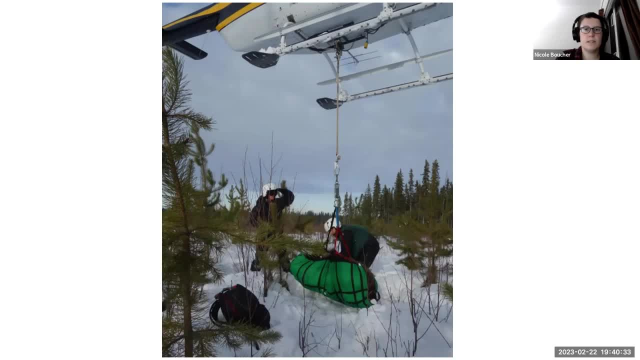 calf body weight between surviving and non-surviving calves. so a subset of calves were weighed by helicopter. however, sometimes it's pretty difficult to actually weigh the calves, so, for example, if they're in a forest habitat, you can't actually get in there to weigh them with the helicopter. 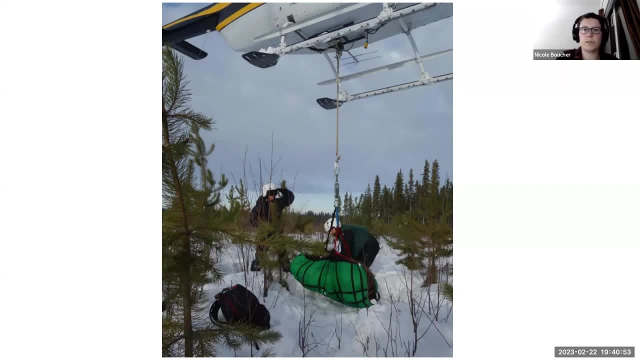 so we used an estimated body weight for this analysis, which was predicted using morphological measurements including total body length, chest circumference and neck circumference, and this is commonly done for ungulates, since they are hard to weigh in the field, and so I compared the estimated body weight between surviving and non-surviving calves. 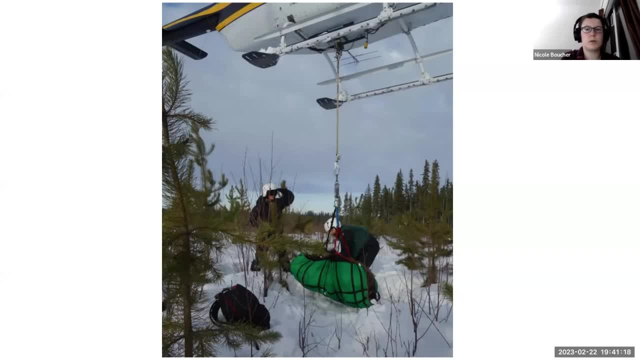 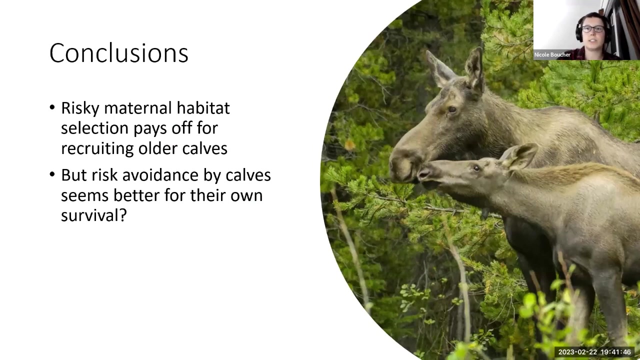 however, I did not find strong support that predicted body weight was related to calf recruitment, with the null model being most supported, and so this is potentially potentially due to using the estimated body weight, but it could also just be that body weight of calves is a poor proxy for their health. so, overall risky habitat selection with forage. 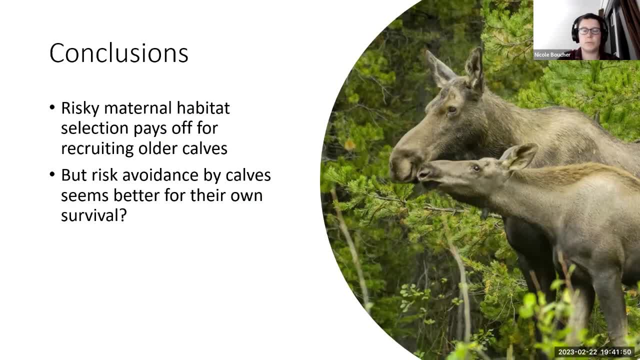 prioritization appears to pay off for mothers in recruiting older moose calves. successful mothers exhibited risk-prone behavior with selection for polygonal disturbances. at that, increased forage likely bolstering energy allocation offspring and this likely helped successful moose offset body conditions exhibited in the prior winter caused by energy invested into. 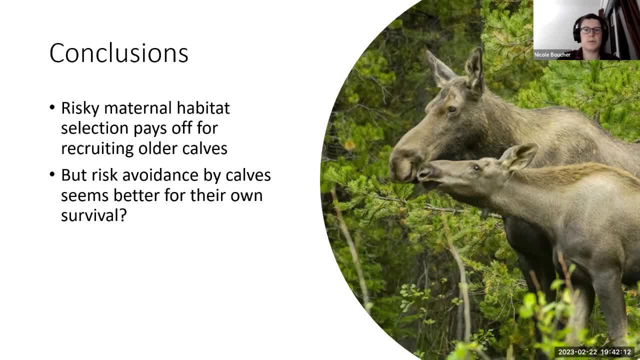 a previous calf unsuccessful female. selected habitat with more five hiding cover but potentially poor forage, which possibly led to less energy allocation to their offspring, especially when considering their higher winter tick infestations, which may have also been present um, which were likely also present on the calves um. so, conversely, um for calves risk avoidance. 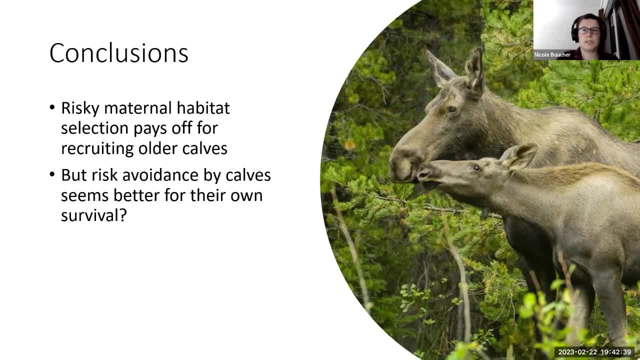 appears to pay off more when examining their habitat selection directly. so calves that survived seem to prioritize use of habitat with more hiding cover and move faster when in risky habitat, and calves that didn't survive avoided potential escape habitat and seemed to linger in unsafe habitat where they may have been exposed to predators. so this difference in 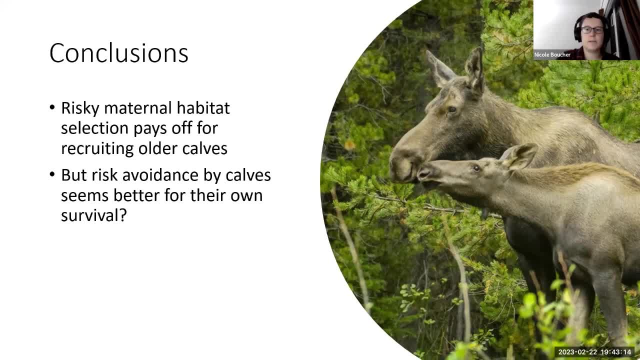 risk avoidance by mothers and calves could be attributed to the temporal scale of both analyses. so for the mother analysis i would be looking at um- seasonal habitat selection, from before the calf was born all the way up to um, when the calf was one year old. so they could have been making riskier decisions earlier on that. 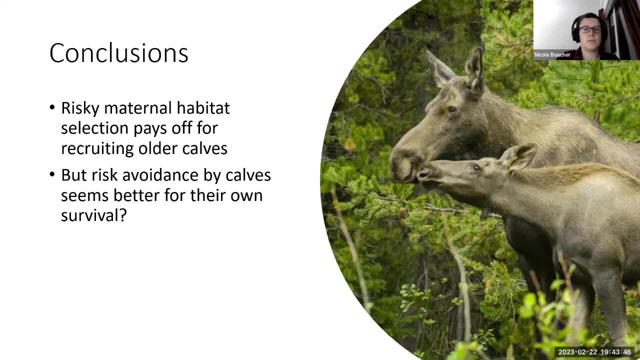 allowed them to supplement their diet with forage that they needed to keep their calf alive, whereas later on, when they're calf, um was um present, um the the calf. um avoiding risky habitat? um for the calf, avoiding risky habitat would pay off more um. it also is um important to consider that each animal is making. 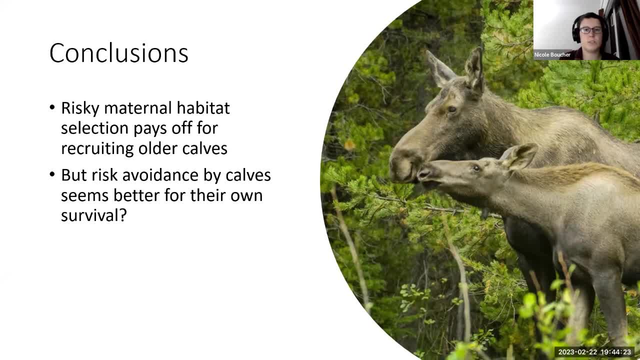 uh, decisions that maximizes its fitness more so than um necessarily, what its offspring are doing, um. so the mothers are always attempting to maximize their net fitness, which means that they could be trying to recruit to their current calf, but they could also be prioritizing on staying alive and reproducing in the future if they think that their current situation uh. 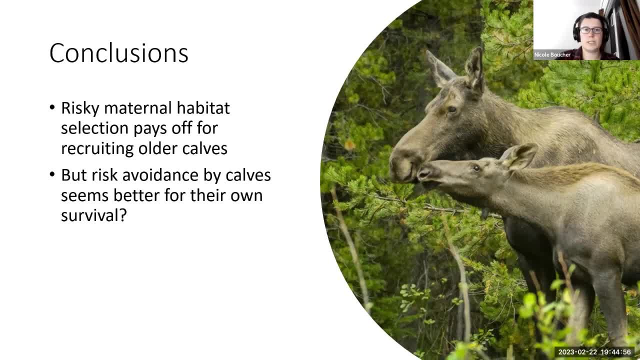 is just not um conducive to recruiting a calf such as if they're in poor body condition um, whereas a calf um or a calf avoiding risk is quite important because they are so vulnerable to predation um. so, overall, these results do highlight the importance of spatial complementation of high 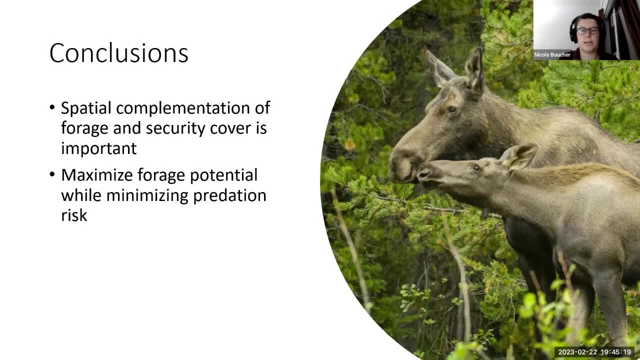 quality foraging habitat and hiding cover for older calf recruitment, so to support most calf survival. uh, this is just a quick summary of the results from the um management report, which is the one that is most popular as far as baltimore is concerned. so, um, we hope that you can find out how to properly manage your calf and your cubs using these results, so that you can give us a quick summary of the results, of the results we're 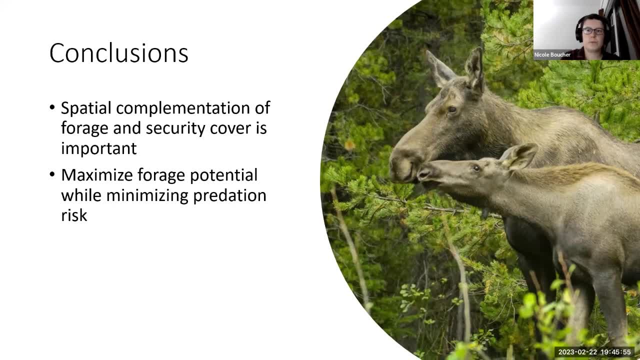 features into previously inaccessible areas or areas with a high forage potential should be minimized, And linear features that link cutblocks should be deactivated in a way to impede predator movement and reduce predation risk across the landscape, And cutblocks should also be designed. 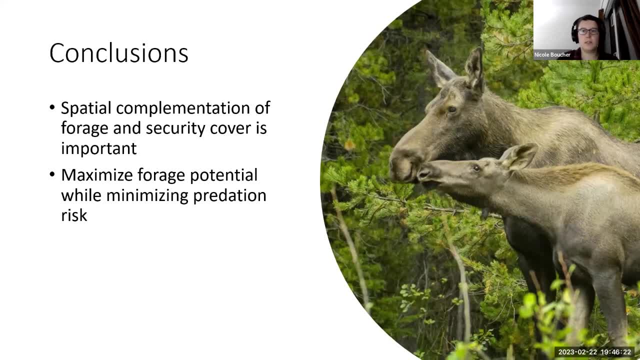 to maximize edge habitat, which augments forage, while also minimizing predation risk, with interspersion of mature forest, which provides security cover. And then as well, if cutblocks are replanted, there should be deciduous vegetation included, withstand tending practices that minimize forage, such as brushing, minimize. 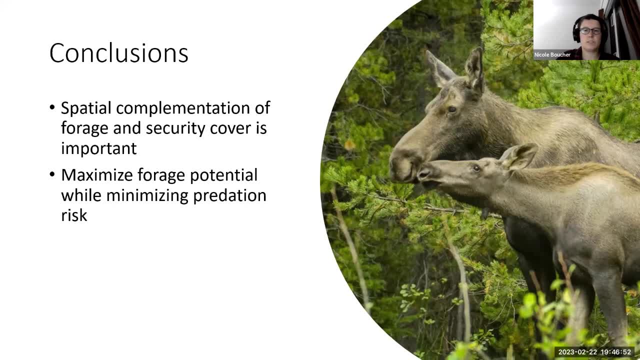 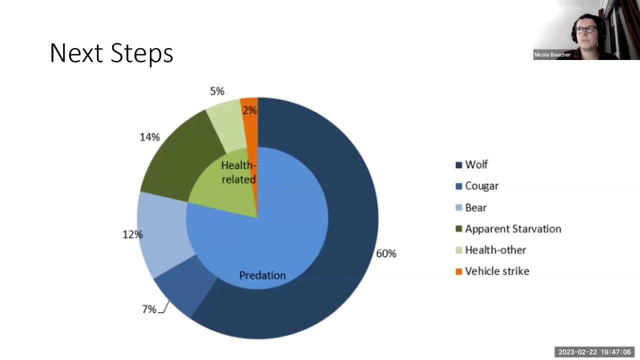 tending practices that minimize forage, such as brushing minimize to promote forage, which is important for calf survival as well as future reproduction of cows. So I'm just going back to this graph to wrap up. So, as a reminder, most moose calves in this study area did die from predation. 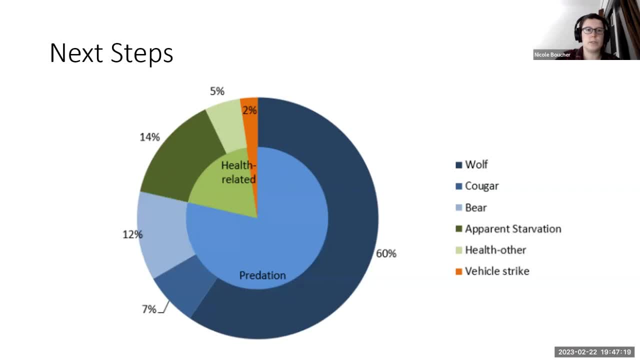 However, while we do have lots of data on what the predators are doing in our study areas, there's a more limited understanding of what the predators are doing in these landscapes, And so a lot of the evidence- that of how predators do use landscapes- has come from other regions, and there's quite a bit of evidence that predators and other animals do. 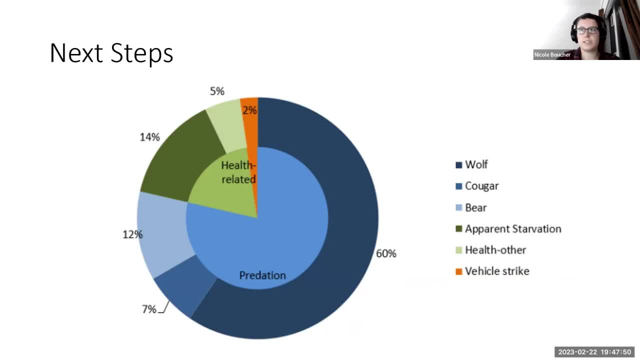 vary in how they react to predators respond to disturbances between landscapes. So the next steps for this project are to look at how the predator distributions are being affected in the landscapes by logging and other anthropogenic disturbance features. So to do this, we have camera traps. 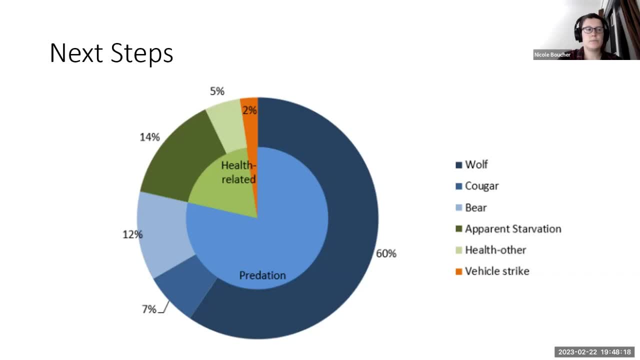 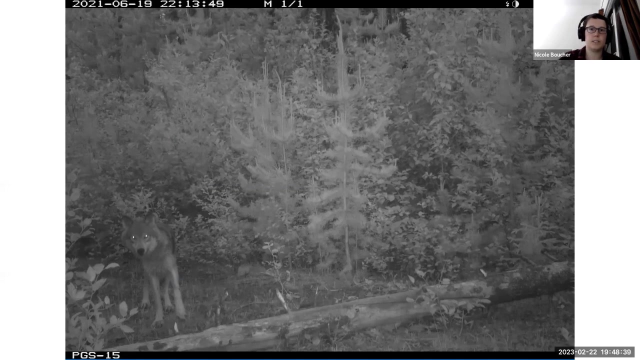 that we've deployed in Prince George last year and currently have cameras out in around the Bonaparte Plateau looking at the predators that are in the area. So things like wolves, black bears, grizzly bears and cougars we're focusing on. 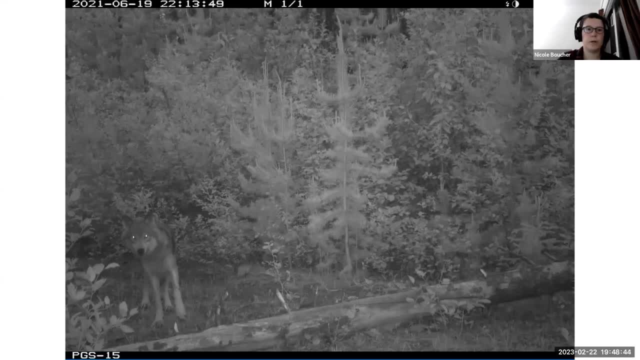 And using the data from the camera traps to better understand the spatial distribution of these animals As well. this data will be used to look at survival analyses of the calves to see if the way that they are using the landscape is non-ideal, which is contributing to their reduced survival. 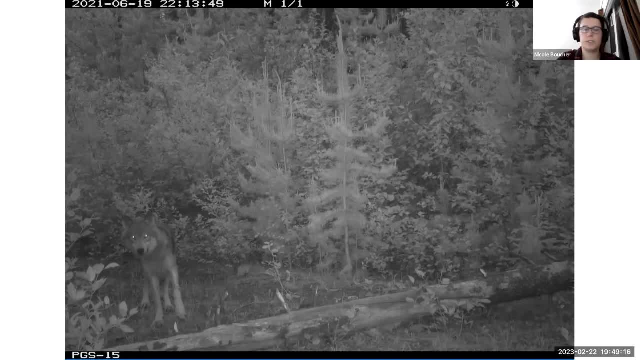 So hopefully this work will be completed within the next year, So keep an eye out for that as well, And so keep an eye out for it. And then the habitat selection work that I did present is currently going through the review process, So keep an eye out for that as well. 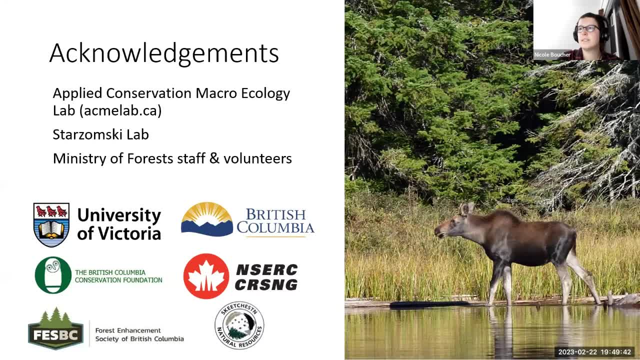 So just acknowledge everyone that has helped with this project or supported this project. There is an ongoing increase in my interest, which is a lot, So there is a lot of work that has to be done, been a lot of people that have contributed to this work and it's a lot of work that has gone into it. 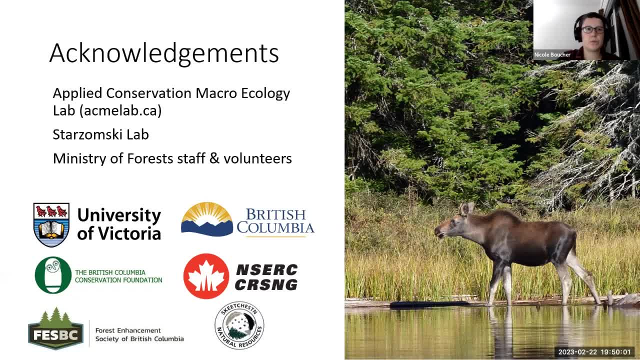 by the ministry of forest, staff and volunteers in capturing and managing the huge data set that we've now accumulated, as well as all of our funders i would like to thank, as well as my labs at the university of victoria, dr jason fisher's lab and dr brian starzomski's lab. 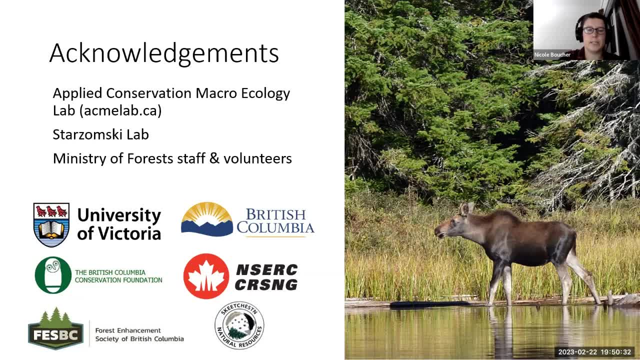 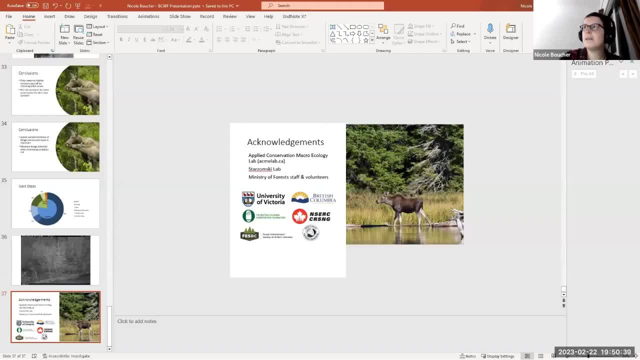 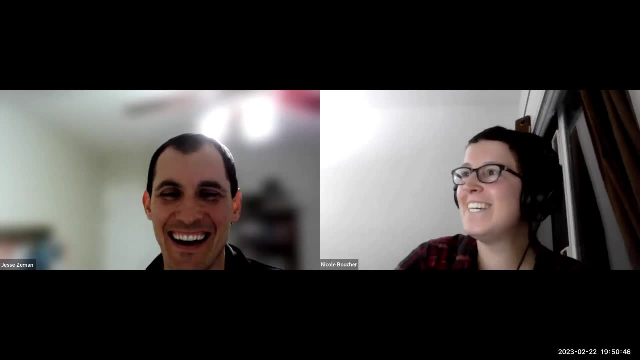 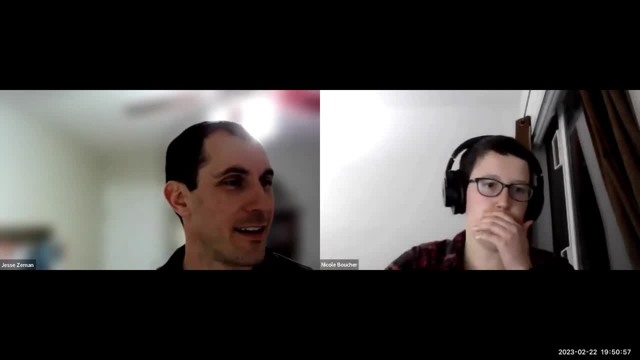 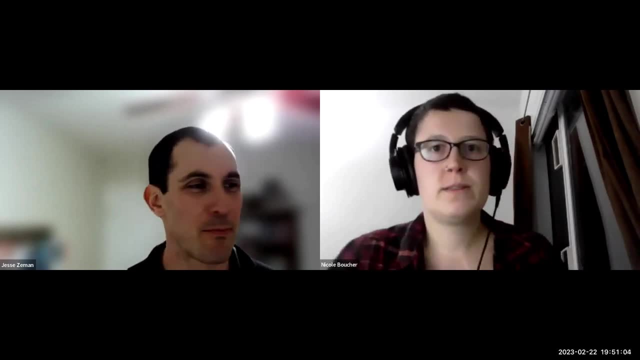 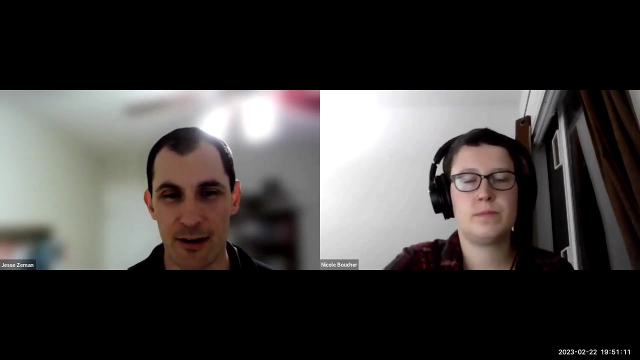 questions that we have here, and i think i'll. i'll deal with a few of the themes to start out, and one which is probably not going to be a surprise to you: um, but are you able to talk about the bearing of monoculture replanting? um, and i don't know if you've done. 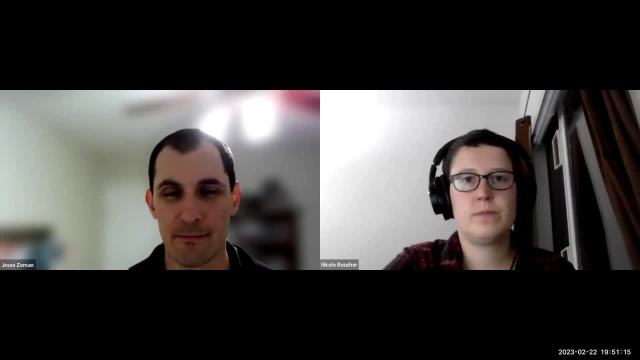 did you do any work related to glyphosate and um spraying in your work, or have you looked, done any comparison between areas? so i guess the first one is: have you looked at the monoculture issue and have you looked at spraying? i guess would be the questions that are going to come. 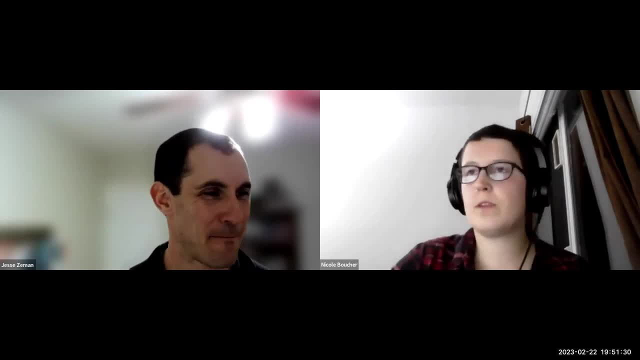 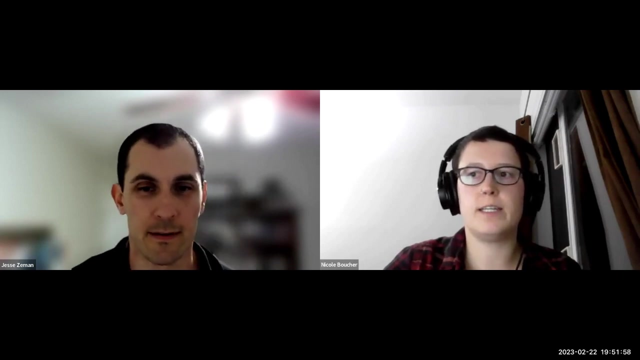 up multiple times um so far i haven't looked at the? um monoculture or herbicide too much. my focus has been more on predation. um also the way that the habitat selection analyses worked um they? um weren't as conducive to looking at that um. i'm kind of hoping that i can. 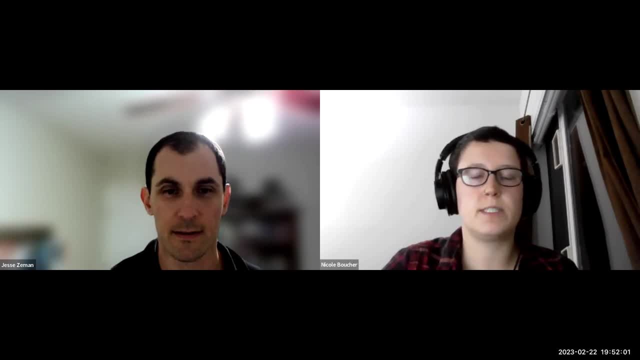 incorporate it more into the survival analyses because i will be able to look at more of a home range um side of things, which will allow me to better incorporate those measures into the model um. but yeah, currently with the, the habitat selection analyses, i haven't looked too much into that. okay, awesome, thanks, um, and you, you may. you, you touched on the problem, but 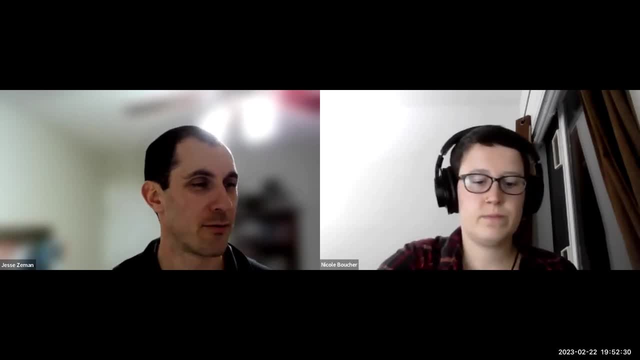 uh, one of the questions is related to linear features. does the removal? is there anything in the lit or off the top of your head around the removal of linear features having a positive impact on moose populations and calf survival? um, yeah, there is. uh, i mean the moose um. 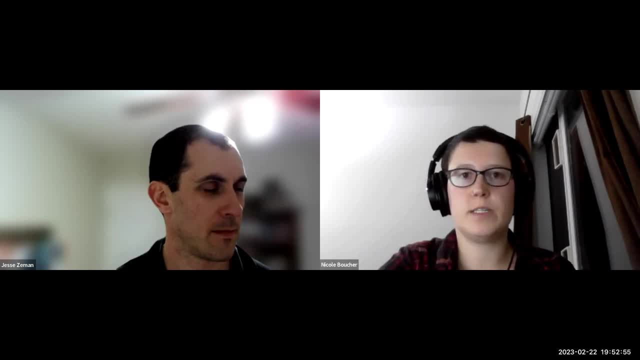 a lot of the work on linear features has been related more to caribou um, but with moose there is evidence that they, when the the linear features are restored, they aren't impeded by the um restoration work as much as by predators are um, so they would. 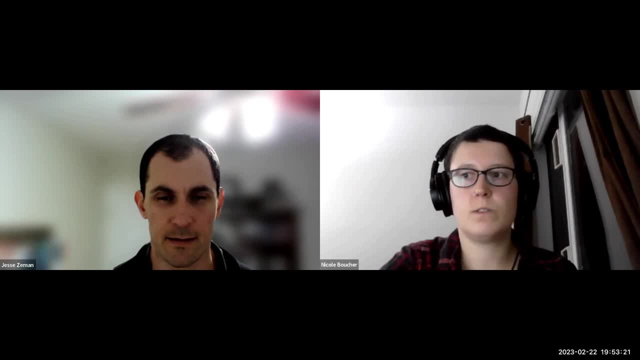 do better in, uh, this area where there's restored linear features, um, i'm not sure if i've read any specific papers that i can think of coming off top of my head where it's had like a population level impact, um, but definitely in terms of movement and and. 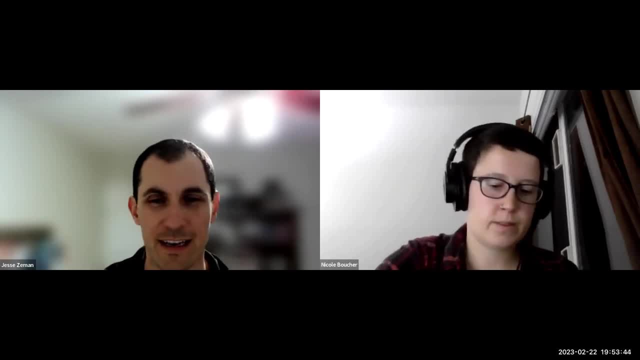 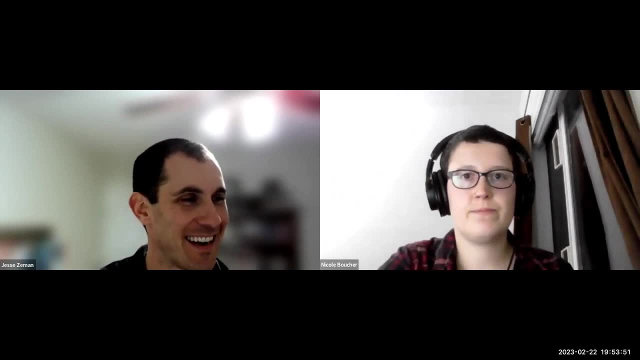 predation- okay, cool. so there's disproportionate benefits to restoration- okay, um, here's a kind of a theoretical question: if you were to create the perfect moose habitat, what would it look like? um, i think it would be a habitat that isn't uniform. um, because they need. 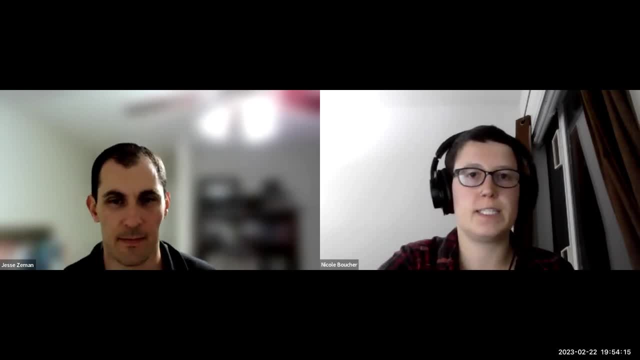 um a mix of a lot of different things to survive. like they need to have the wetlands so they can get proper minerals and nutrients. um they need to have the mature forest to have hiding covered and um to provide good calving habitat. um they need edge habitat. they. 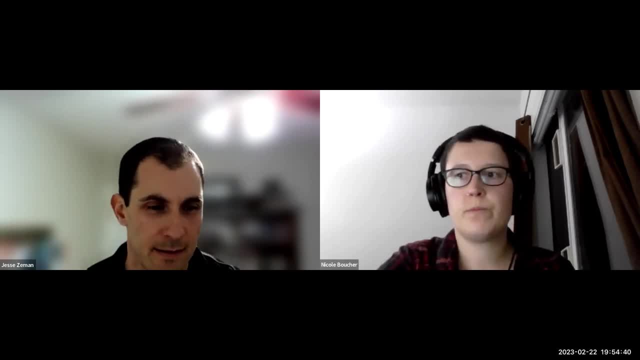 just need um. they need a mosaic of of landscape features, um, not just kind of a, a uniform um have a landscape. and also it does depend on on the region, because it did seem that with my analyses that it is very regional- um on what landscape features do seem to work better for. 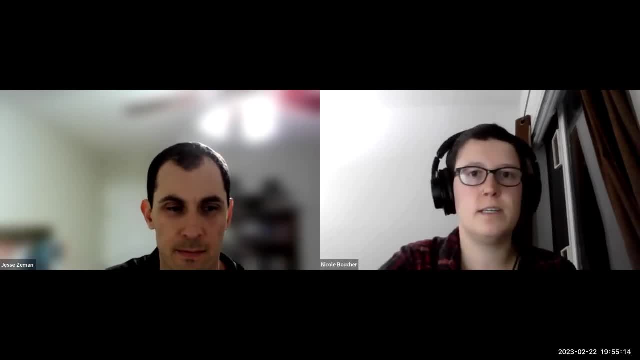 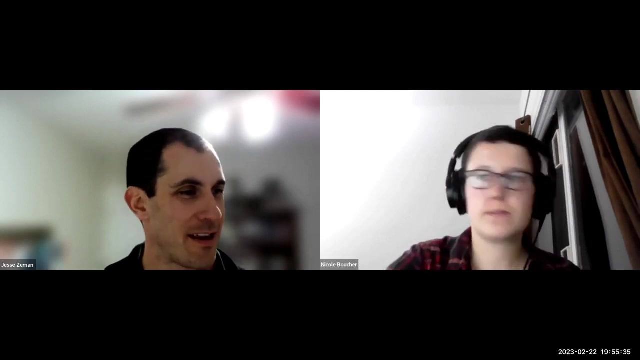 calf survival. um, at least for my focus, um, they did differ quite a bit between landscapes, um, so i think that the perfect landscape really depends on where you're looking, um, what the biogeochromatic zone is, and stuff like that. okay, thanks, uh, this one is gonna be. uh, this is far more specific, related to logging, and you may not. 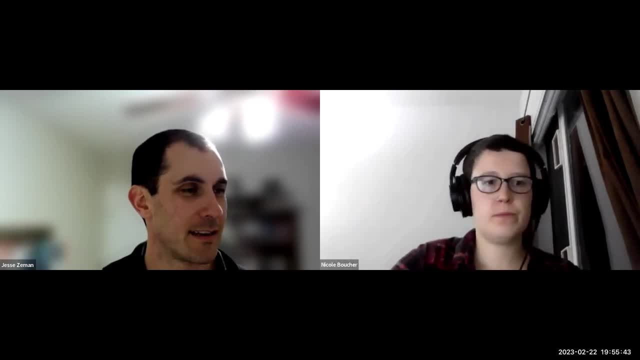 not. this may not be something that you're even able to look at, does it's? uh, the question is: does scarification increase calf mortality? uh, i'm not sure. okay, perfect, sorry, no, no, that makes sense. that'd be a hard one to answer. um, was there any? okay, so somebody's asking correlation. 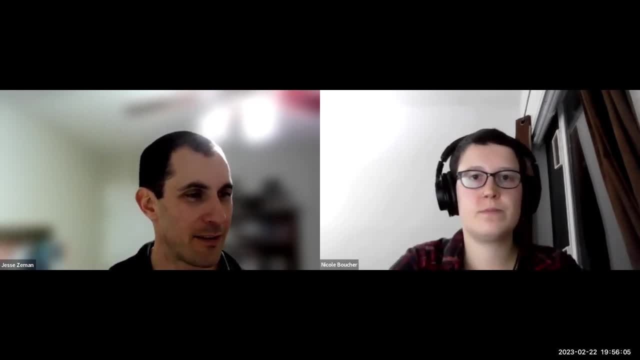 observed between winter tick load preferences for resource and risk avoidance. i mean, that gets pretty complicated. but um, did you layer all that up and look at interactions at all? um, i'm kind of hoping that i can do a better job of of assessing that with the survival. 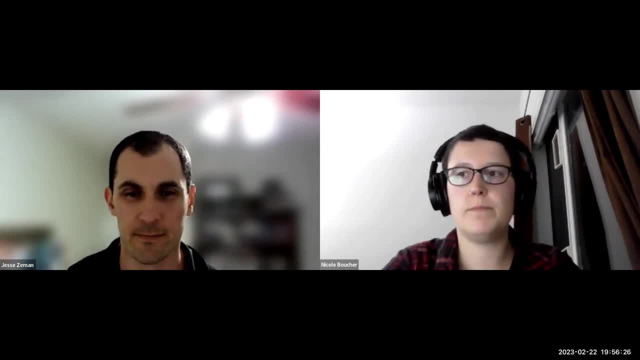 analyses, because i'll actually be able to um incorporate all the variables within the same model. um currently, um the way that the analyses are set up, um there is like an implied relationship between those um, between risky habitat selection and higher winter tick loads, but um i haven't explicitly made that connection yet. 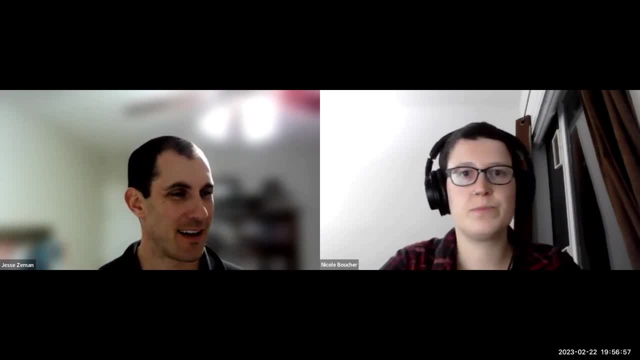 okay, uh, okay. so this question: um, so it says cup blocks provide more browse and therefore food, yet had increased probability of predation, moving more quickly through risk areas but still accessing forage. so i mean that really ties back to your last answer around mosaics and kind of diverse landscapes. um, does the pi chart uh that? 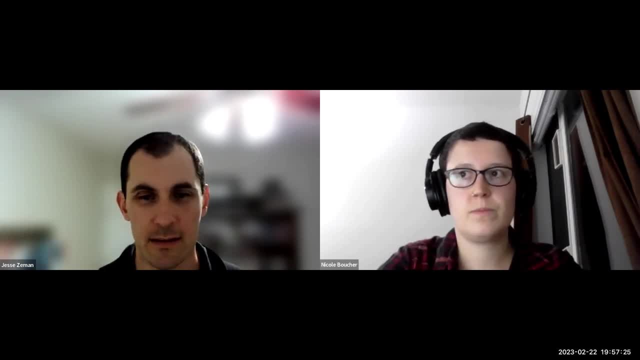 was around survival? was that only for calves? um, more stuff. yeah, that one, that one was calf focused. okay, and how does that compare to cow? um, warts, um the cow. mortalities are a little bit more diverse because there's there's like hunting and and the. 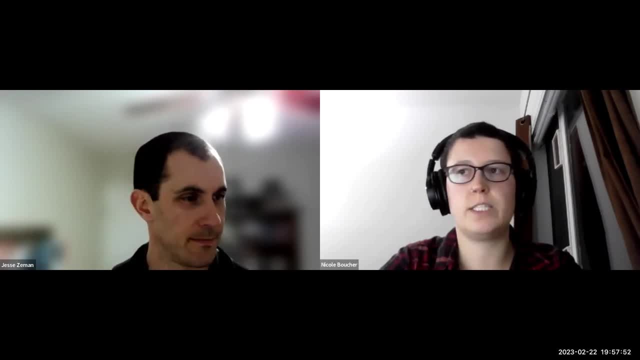 calves: um, the the pie chart for the calves is focused on uh, before their first birthday. so, um, it is very like predator heavy um, but there is still quite a bit of predation for the cows. awesome um are, is any uh, are you doing any work in the big creek area? so that would be west of. 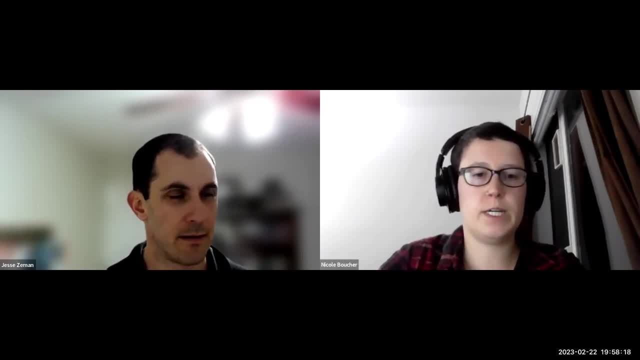 williams lake, um. my study area spans kind of from um cam loops to 100 mile house um and cash creek area kind of all in that area. yeah, yeah, there's big, there's big creek is included in there. yeah, yeah, there are callers out there, okay, um, so you had ultrasounds, oh, what was um fecundity? what were kind of pregnancy rates? 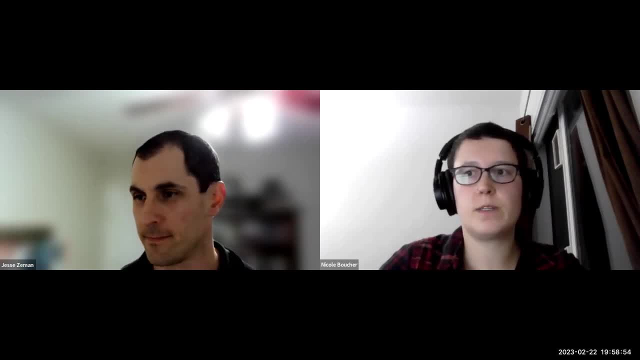 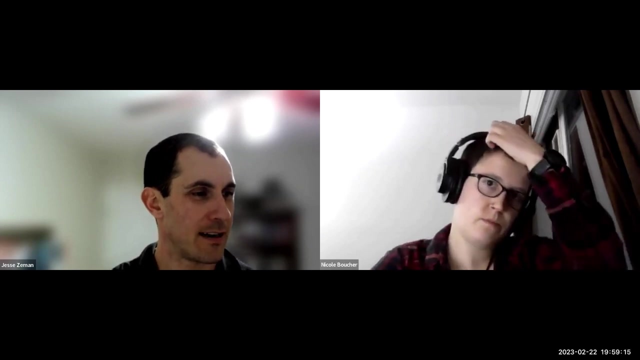 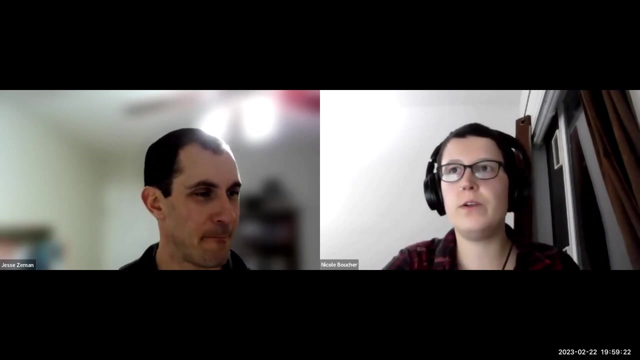 look like, um, the moose are pretty much there's, they're really high. uh, most moose are pregnant every year, but they're they actually. yeah, that's good. uh, you link calf recruitment to cows. being previously successful with rearing cows the year before, was this care? was this compared to the age of the cows at all? so, yeah, no, i didn't. 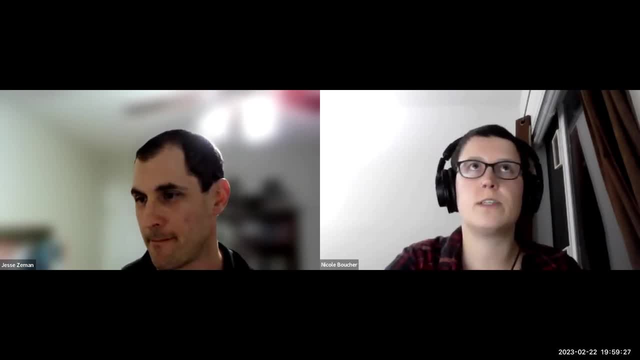 compare it to the age of the cat at the age of the cows, um, i suspect that it would have um an influence, but we had a limited sample of cows that had been paired with a calf that had also been captured the year prior um, so i wasn't able to. 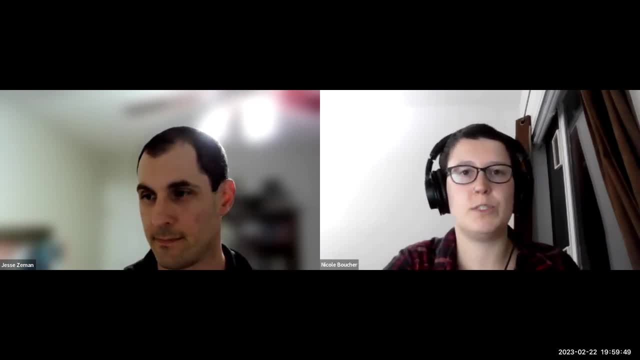 go into that depth with the analysis because of the limited sample size. awesome, uh. another question: any evidence of coyote predation on uh cows or calves? um right for for our work it focuses on the eight-month-old calves, um, so the predation has all been wolves, cougars and bears? um, i'm not. 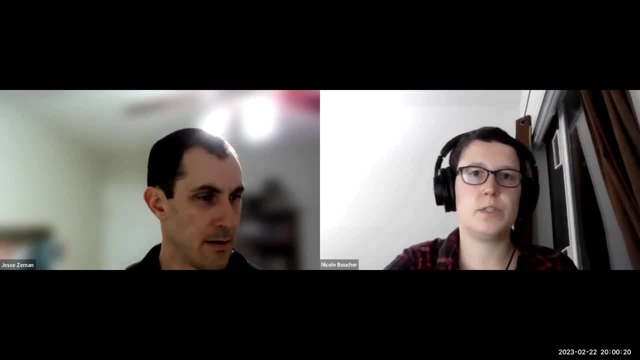 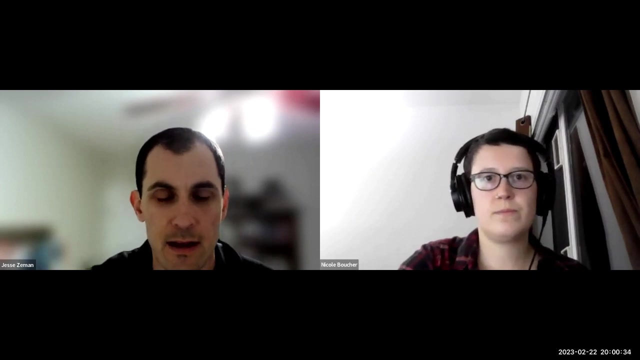 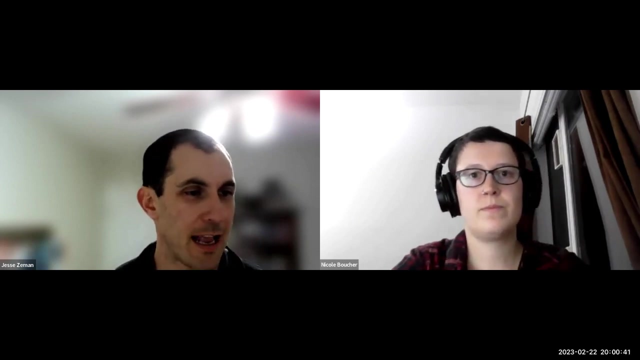 sure about neonates? um, there's the potential, but i don't have evidence of it. awesome, uh, okay, what was the next question? okay, when you do post-mortem investigations on moose, uh, are you doing any sampling for, um, glyphosate in your morts? um, i don't think that they do. um. 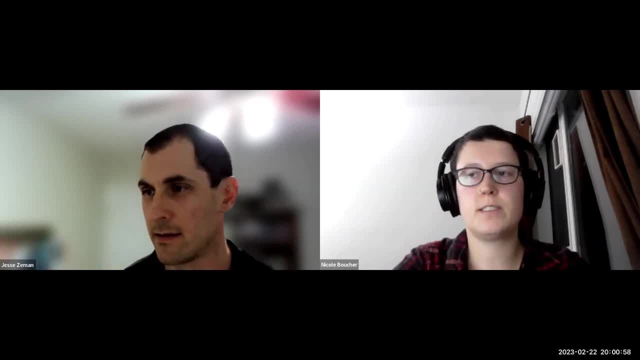 i think that we mostly are looking at parasites um body fat, um, like from looking at marrow fat um evidence of predation or the predator that was involved, um, um and taking like samples, long bones and stuff. i don't think that we really look at um herbicides. 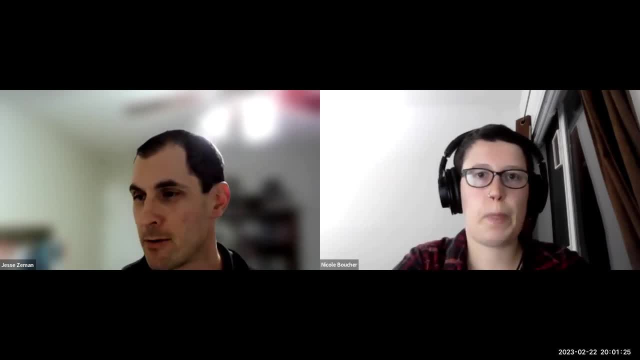 okay, awesome, um, okay. so this is background edge habitat. it really it talks about how how much salvage is really going on and i guess, um, you know, in those areas it's a lot of information, um, and i think that's a good point, because i think that's a good point, i think that's a good point. there enough hiding cover left and what do we need to do to ensure there's sufficient forage on the landscape as these things age, i mean. so really, it comes down to what are your recommendations to try to restore or reduce, minimize the decline in these areas? as it relates to how the landscape 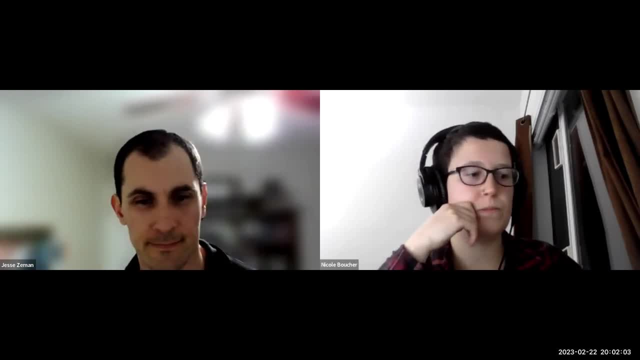 is being managed. i think that the way that we are going in and logging everything that has um, like the salvage logging i don't think is always necessary um. i think that it is important to leave some of these stands of um and mountain pine beetle infested trees um to leave the the diversity in the landscape. 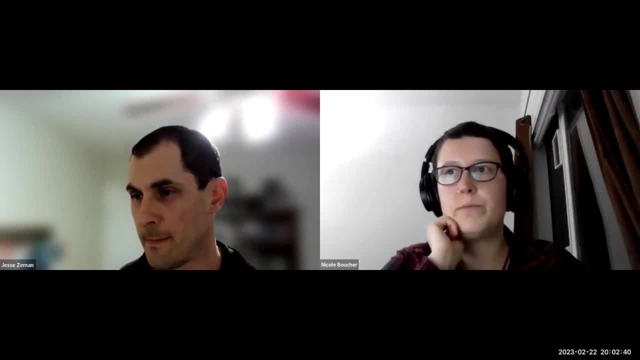 um, because currently, right now, the? um the cup blocks that are in the landscape are quite massive, at least the ones that i've flown over. um, i think that just the way that we look at disturbances needs to change: the they're not something that we need to go in and clear out um, all of kind of the, the deadwood. 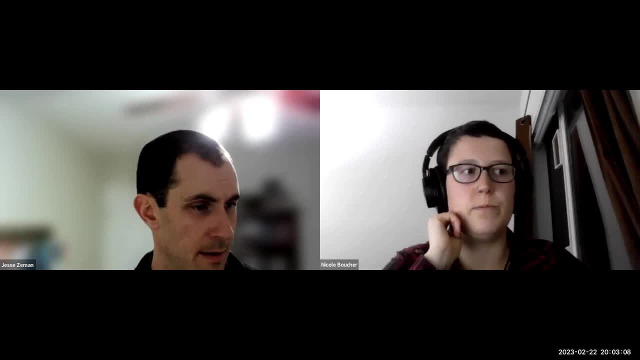 um and and um understanding that we do need to recover some of that timber um so that um the economic value is retained. um but also letting um the market with mountain pine beetle infested timber does have consequences as well. Um, I think that um. 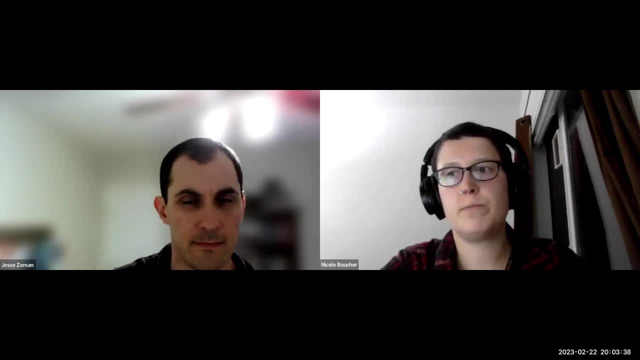 we need to prioritize um treating the landscape um as a natural place that does have the variability um and not managing it um by removing deciduousness, Or um. planting tree monocultures is important um because it is the diversity that has led to. 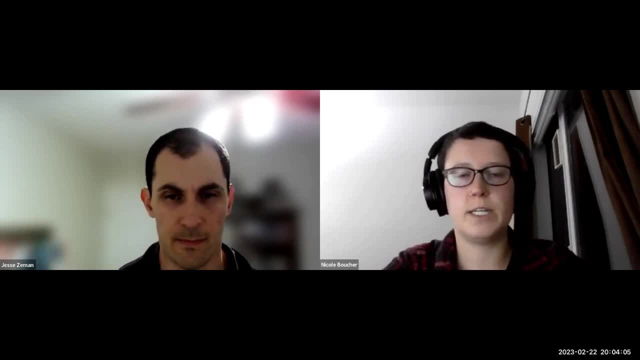 the um diversity that we do have in our landscapes right now and it is important to maintain that. Thanks, Um, okay, so this is around how you- I guess you're cleaning your data. The question is: are there extreme outliers incorporated into your data or have they discarded? I don't know. 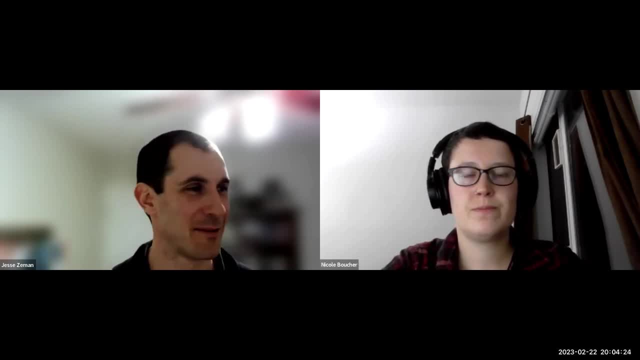 how, how much of a rabbit hole you want to go down and how you manage some of your collared animals. but maybe you can do that. Um so, um, I think, um, I think it's important to maybe a bit of insight, if you have some. 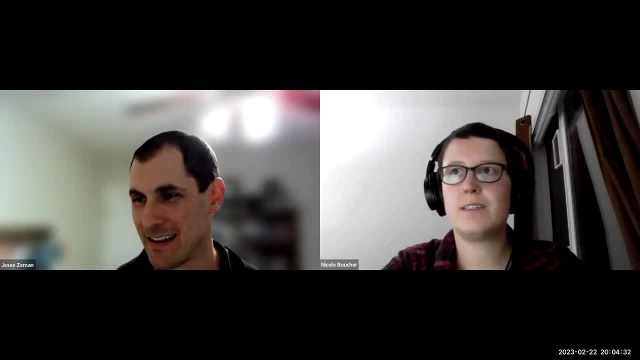 Um, I guess it. I don't know if they had like a specific analysis in mind. Um, I try and retain everything that is within like a realistic bound um and um, trying to think if there's any severe outliers that I have removed. but I I guess, I just say I do. 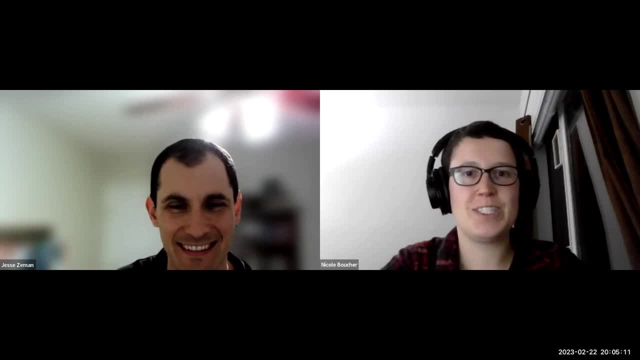 the normal data exploration and modeling process and yeah, Okay, thanks, Um, okay, so, and this is, I think the cameras might help get you there. but last question: is there a direct correlation between predation rate and predator? 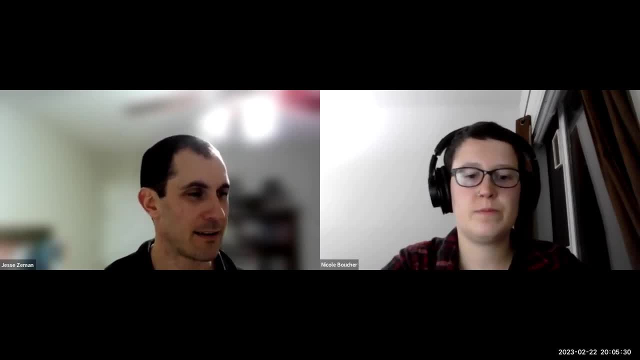 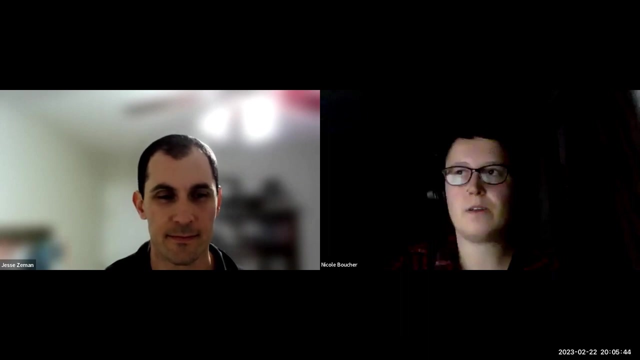 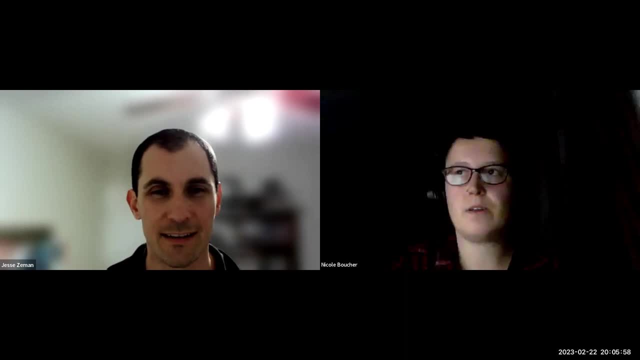 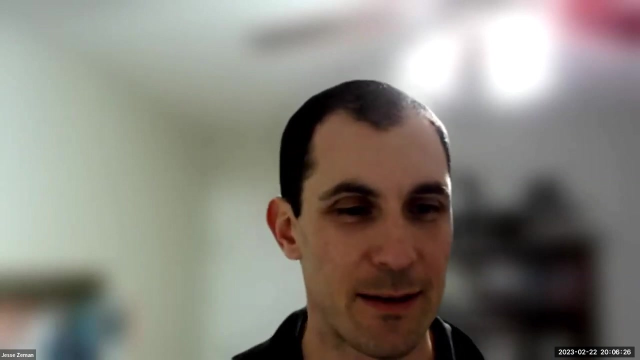 Okay, Okay, Okay, Okay, Okay, Okay, Okay, zoom might have crashed, unless it's my zoom. it's like, unfortunately, nicole's zoom has crashed. yes, okay, well, it's just after eight, so we'll just give it a minute or two and if she gets back, 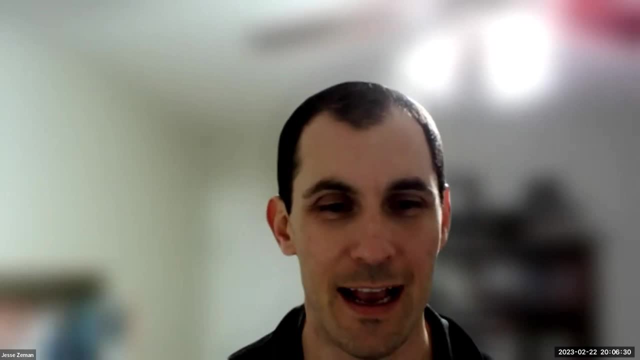 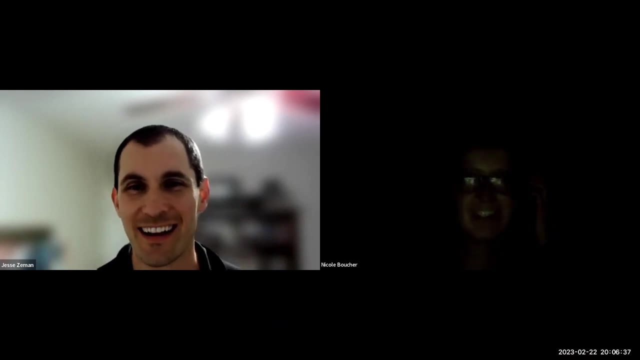 on. we'll continue on with questions and if not, we'll have to call it a night. here we go. she's back. there we go. hi, did the power go out there? yeah, my power just died. we've been in a windstorm all day and i guess the power just went out. 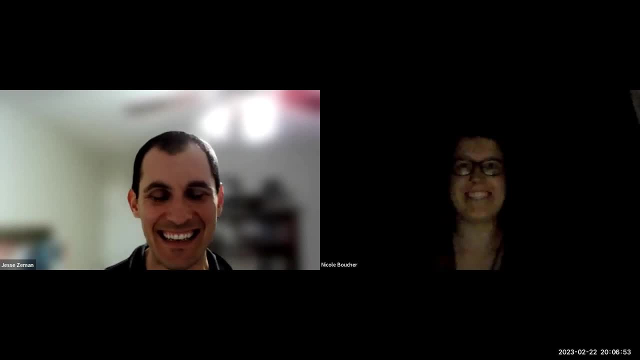 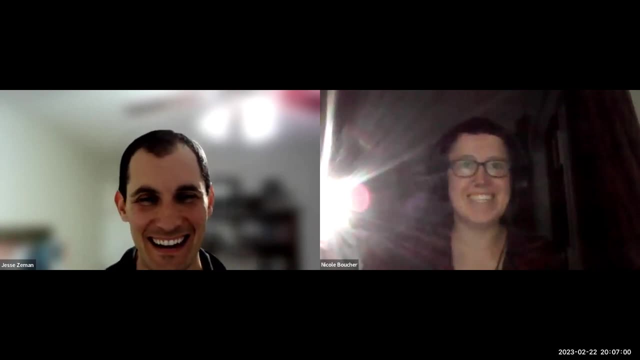 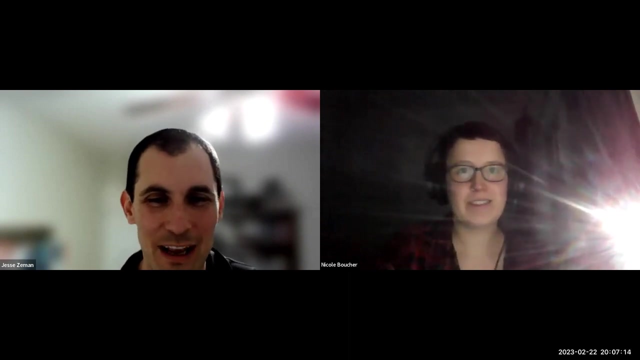 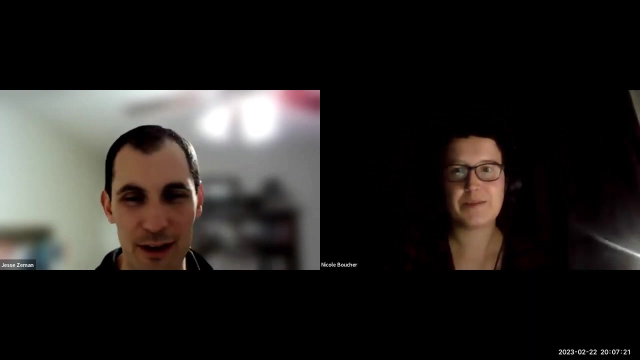 okay, yeah, this is as good as i got. oh, that's awesome. no, no, that's awesome. um, oh, we got you back. okay, okay, yeah, i there we go. um, okay, made it through the presentation. yeah, i'll just check your speed. um, so the last question. i don't know if you caught that one, but it was around. 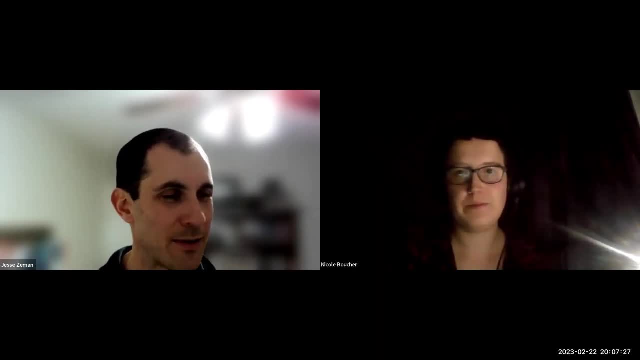 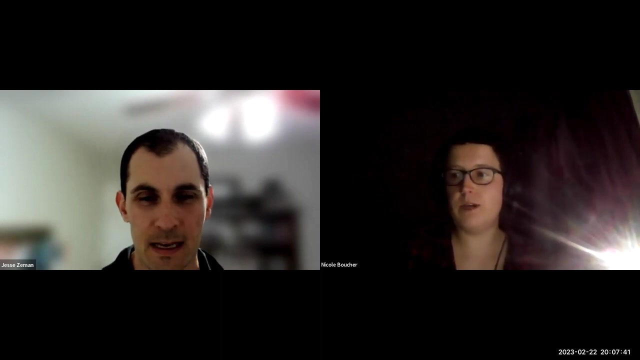 um, essentially, is there a correlation between the predator abundance and the predation rate, and what declines or a decrease in predator populations actually result in a functional response in moose populations? um, i think that i'll have a better idea when i have the um camera trap stuff. 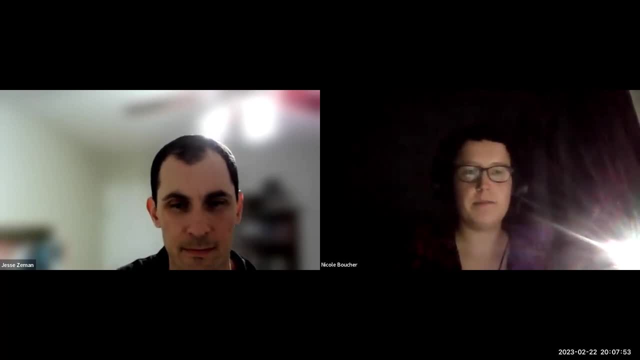 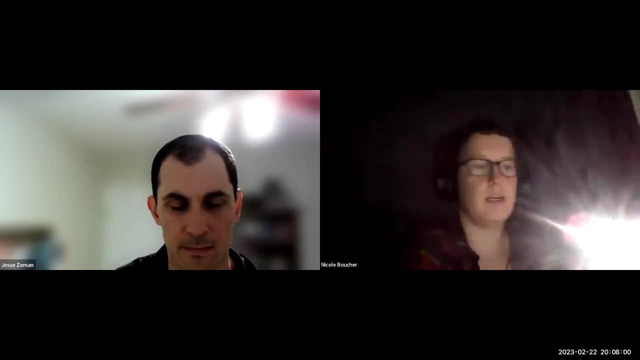 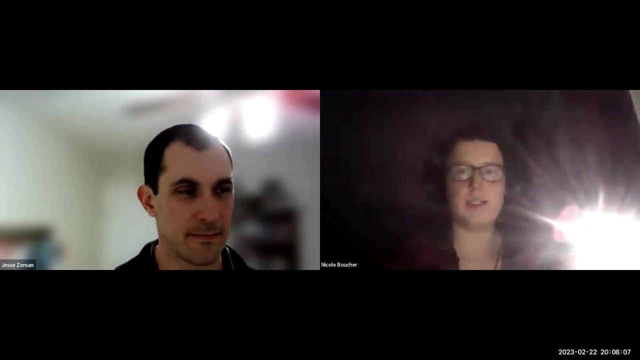 done, but, um, right now i don't think we have a good idea of the predator populations in the area, so it's hard to actually make the connection. um, perhaps i will be more so able to look at the distributions of the predators and not not quite have the 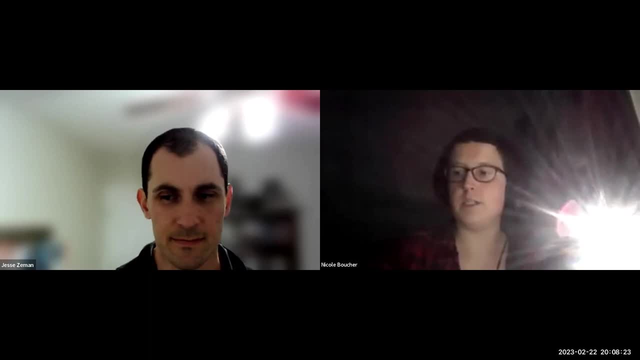 population of the predators, quite as figured out um. just because of the limitations on the data, um, i think that um a decrease in the predator populations would likely um contributes to an increased population of um moose, but um i the predator population is a等倨. 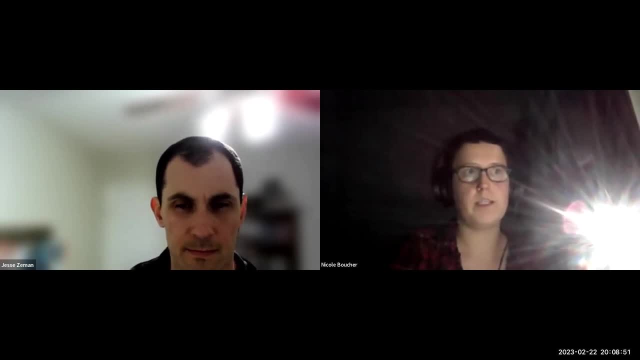 соп 이런. If the predators are still able to hunt quite efficiently through the landscape, I still think that they will be able to keep most populations down, And I also think that removal of predators or decreases in their predator populations and landscape would have impacts on other species within the areas potentially due. 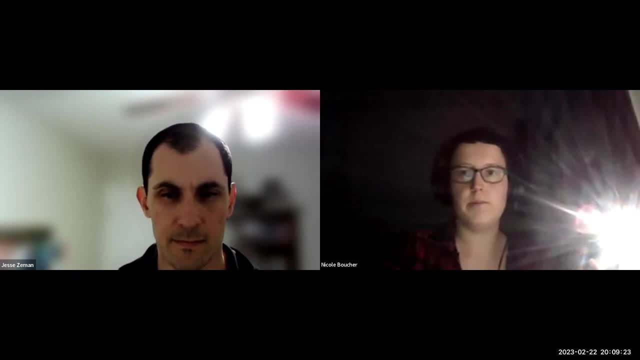 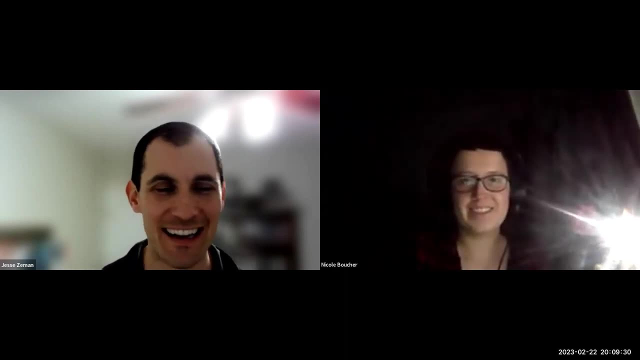 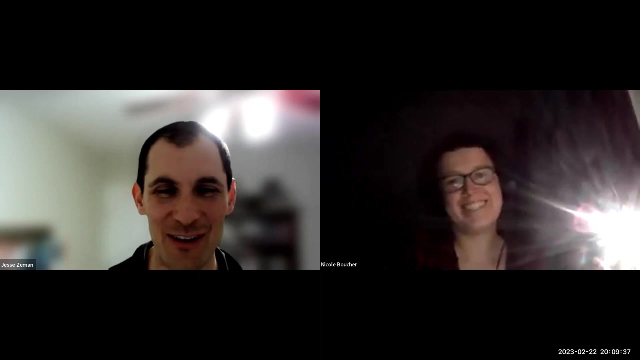 to apparent competition, stuff like that. So, yeah, it's complex. Yeah, Okay, That's awesome. Well, maybe what we'll do, just because you're operating in the dark. so I think we'll call it a night. That was quick. 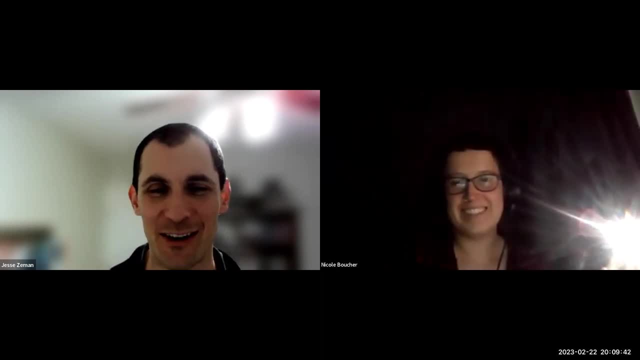 So you're obviously working off your cell phone or something because your internet would have gone down. So that was, Yeah, Hotspotting it, Yeah, Yeah. So that was Really appreciate you coming back on that quick. So thank you, Nicole, for your time. 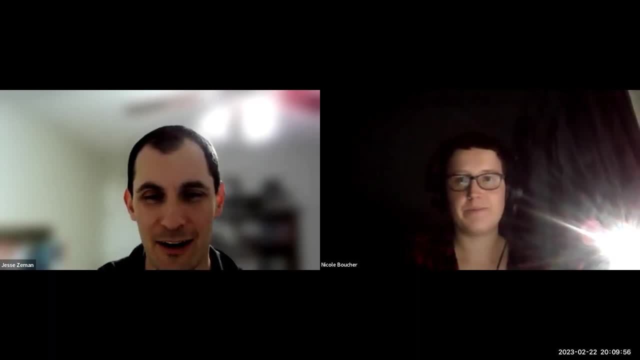 That was awesome. Maybe once you get done and all defended, we'll have you back for the next couple of chapters in the final analysis. So thanks for your time tonight. Really appreciate it. Thank you. Yeah, I'm really excited. Thank you. 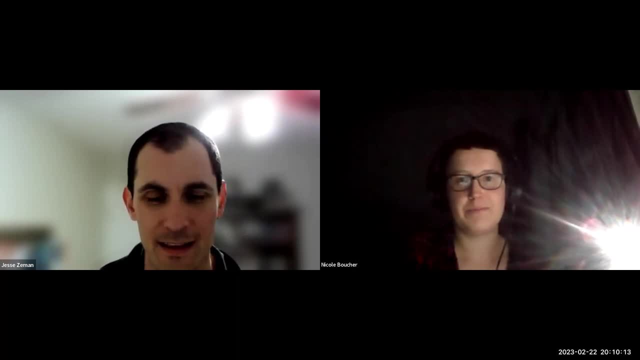 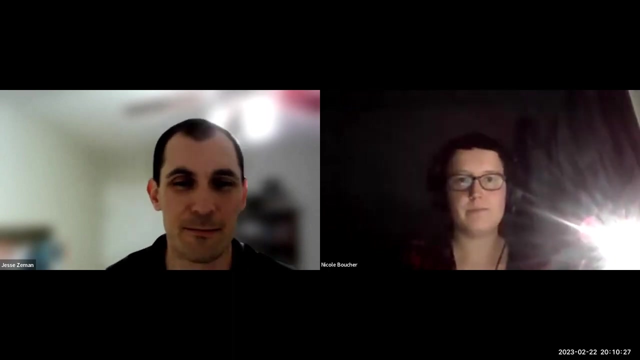 Yeah, Thank you for sharing the camera trap work Whenever it's done. I've been working on tagging through all the images right now, So it'll be really neat to have a better idea. Awesome, Awesome, That's great, And thanks for everyone for tuning in tonight. 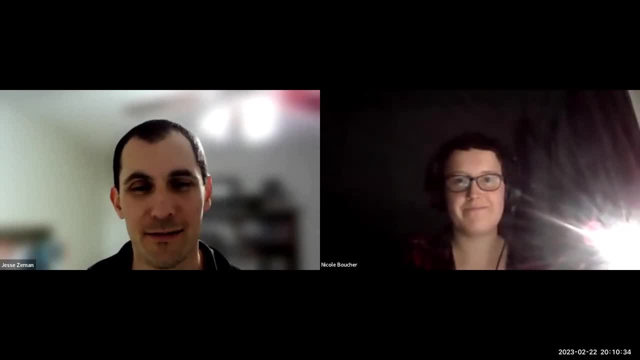 We really appreciate it. I guess the message tonight is diversity in our forests and having a mosaic and leaving some timber in the On the landscape and some deciduous stuff is going to help moose. The next webinar is March 22nd, I believe, with Siobhan Darlington from UBCO on the Interior.